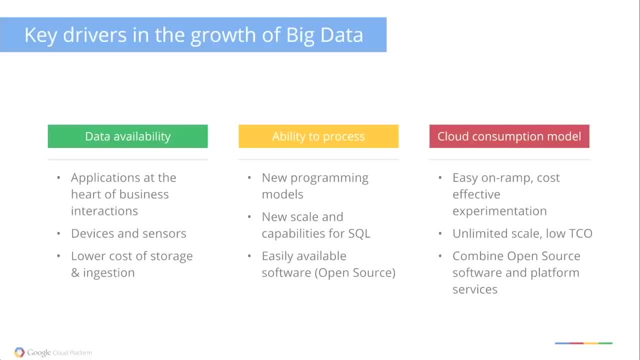 go through computers and programs and generate data, And not just business transactions. A huge number of interactions of all kinds, including non-financial interactions, go through computers and programs And a lot of data is generated that can be kept and help document what happens. 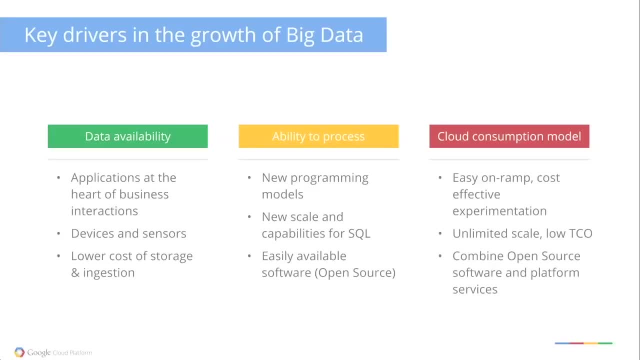 At the same time, there's an ever-increasing number of devices, from cell phones to cars and things like sensors, Objects whose only goal in life is to produce data. That's the issue, That's. the only thing they do is just pump out data all the time. 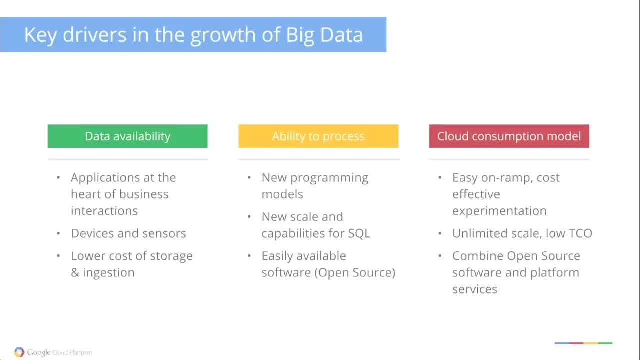 And there's more and more of them every day, every month, every year. Fortunately, the cost of collecting and storing all this data is coming down dramatically as well. So all those three factors together, that explains the much larger availability of data. 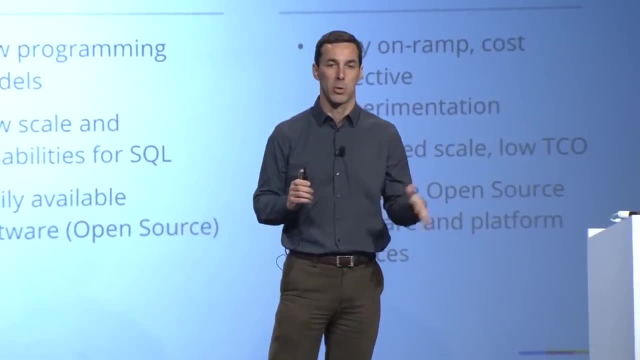 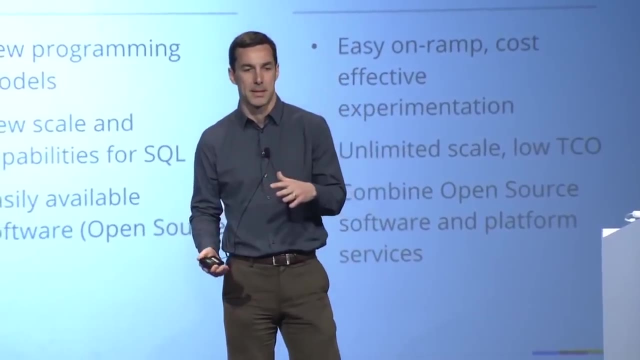 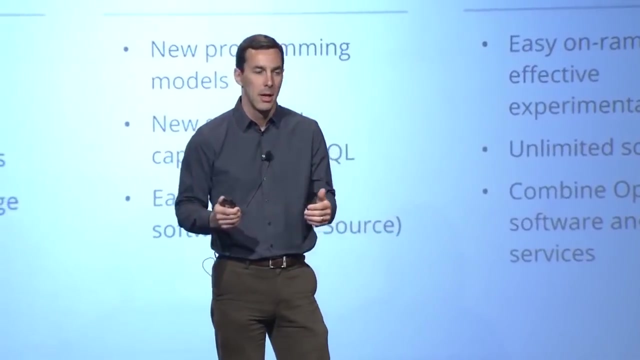 The second widely recognized reason and factor explaining the growth of big data is the increase in the ability to process data at this scale, And these two comes in three main aspects. One of them is the invention of new programming models, The more famously MapReduce, and now some newer. 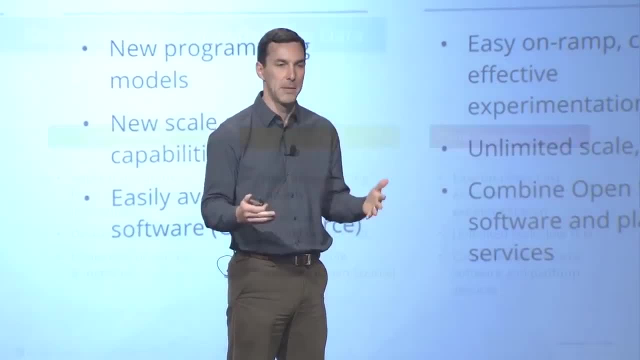 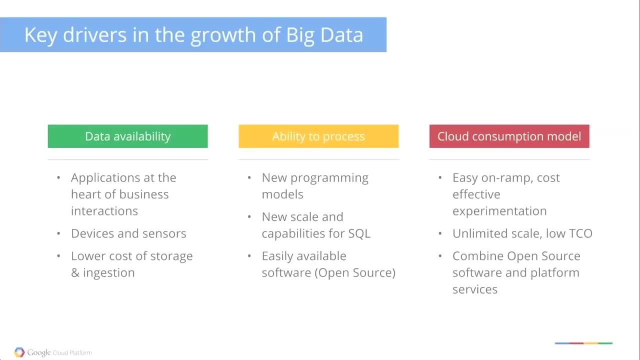 large-scale data processing programming models, which were built specifically to allow people to process data at very large scale in parallel easily. The flip side of that is, in addition to inventing new programming models, we've taken existing, well-known, familiar. 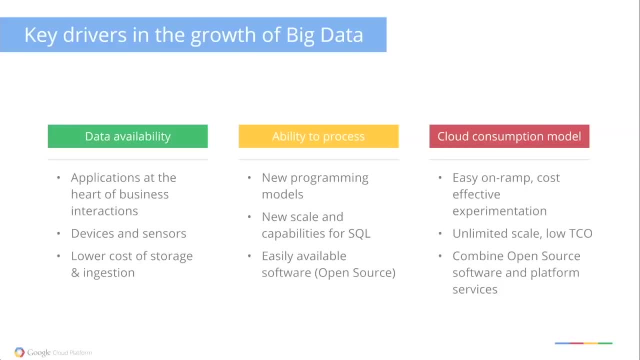 popular methods- SQL, you know, chiefly- and created services that allow those to allow SQL to work at much larger scale and much faster than it was designed to, than it was then to do originally. And then, finally, there's been a huge explosion in the availability of 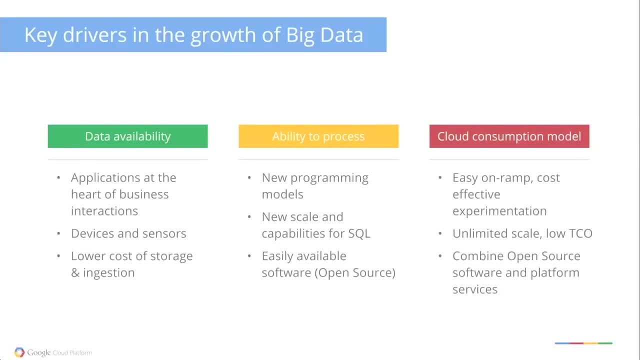 open source software in general, but specifically for big data, And that has really given everybody a wide portfolio of product. they can use High quality portfolio, something that you know with constant innovation, very, very dynamic environment With products like Hadoop and. 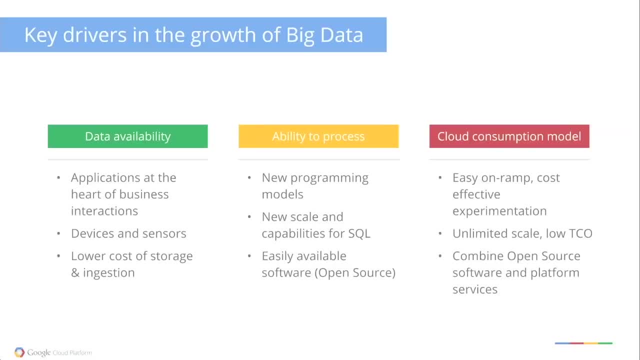 Spark and others, and that has really democratized and brought down the cost of big data. So all those together, that has really improved the ability to process data at large scale. Combining that with the availability of data, these are the two well-understood reasons why big data is really picking up. 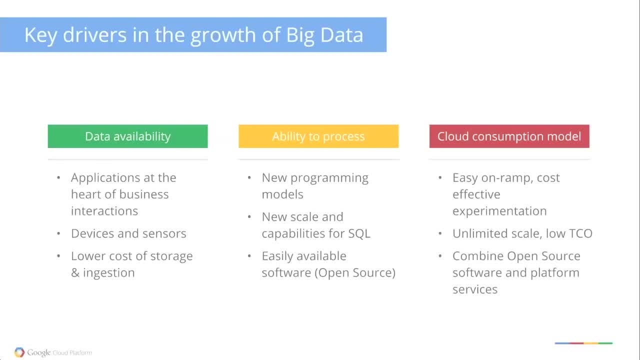 The third one and the one which I would submit is just as important and becoming even more important, and two days in general- and the keynote this morning, I think, has made that very clear- is the emergence of the cloud consumption model for big data. 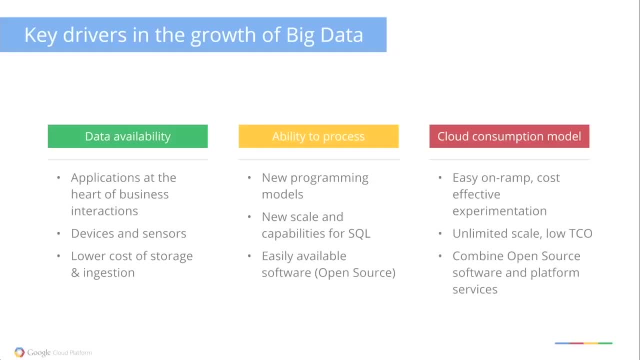 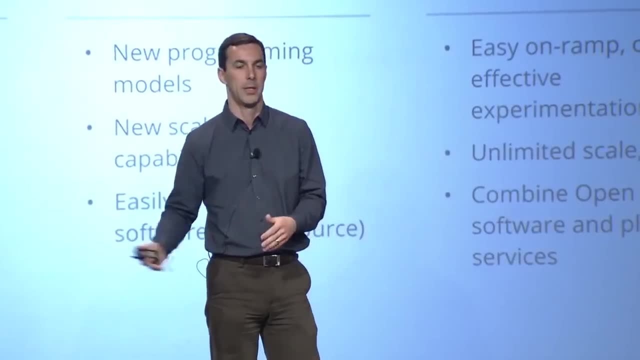 One aspect of that is how easily it lets you get started. You can wake up one morning with an idea and by the end of the day- even if the idea involves pressing terabytes of data, you've tried it, you've iterated, you've tested it. maybe you've abandoned it or you've refined it. 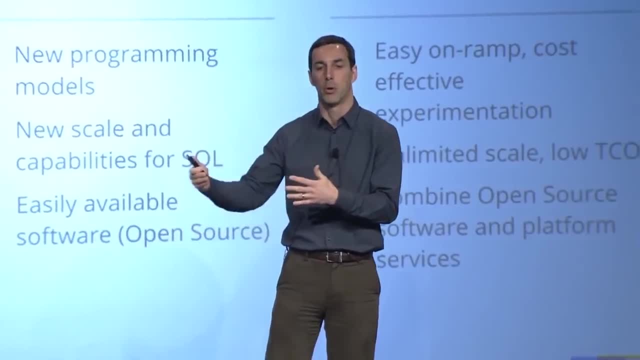 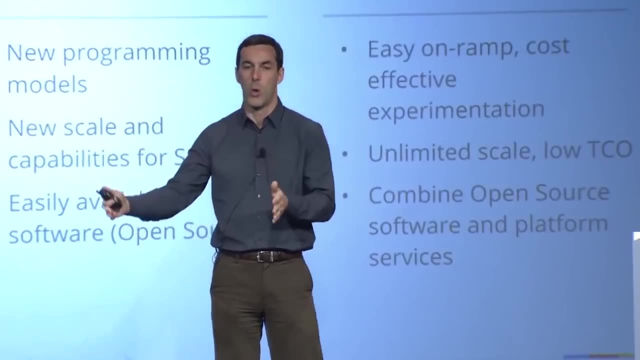 You've already been able to do work with it and make progress without having to start by thinking about: can I do it? What do I need? How do I get the infrastructure? You just go do it, whether it's a one-day personal. 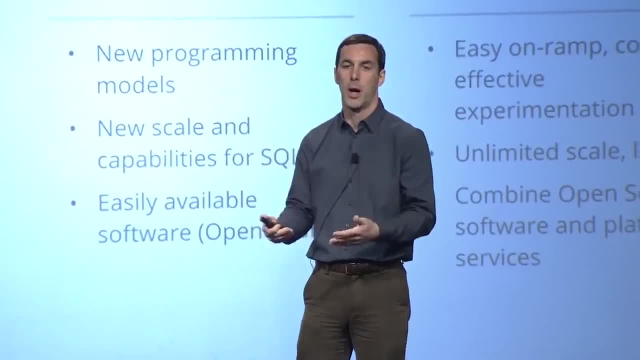 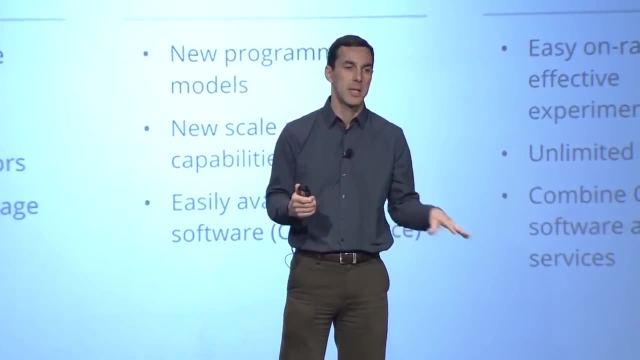 project or a one-week, two-week proof of concept, You can right away start using systems and do that at a very, very low cost. And then for those ideas and projects that actually prove to be useful, that you want to take forward where you are already in the cloud, 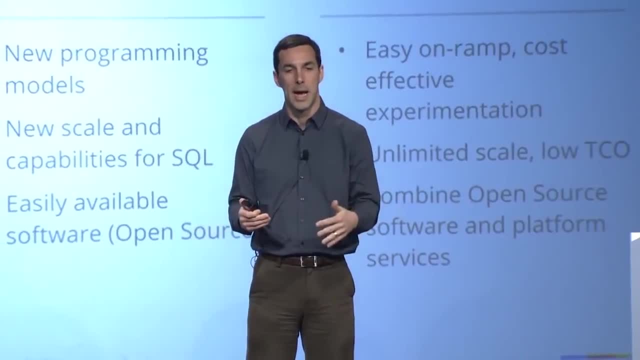 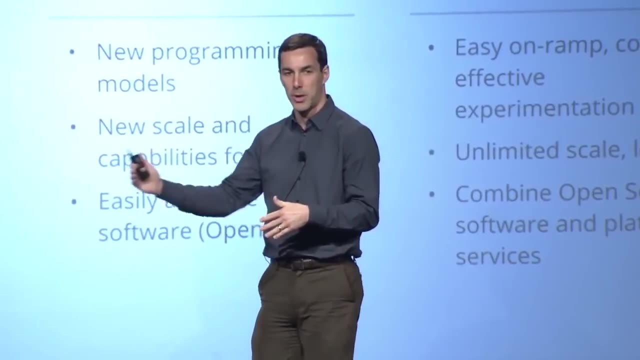 you can scale those pretty much infinitely And keep doing that at a very, very, very low cost of ownership. I think on those, hopefully, you were all here earlier in the morning when Urs talked about the price drops and he made it clear this is not. 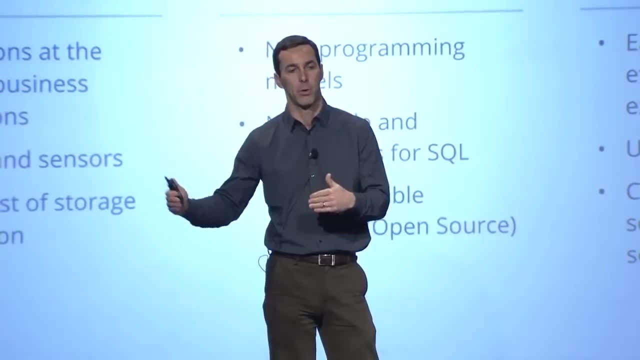 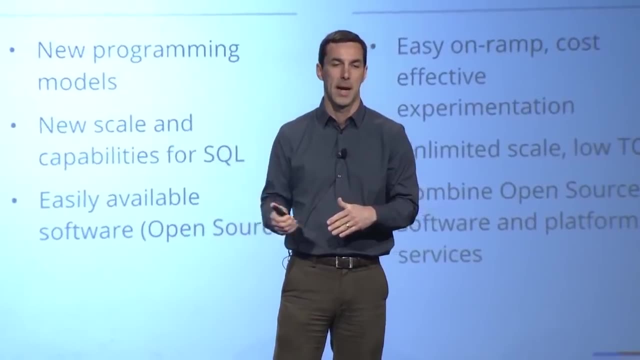 this is not a one-time price drop. This is a continuous effort to really bring the cost on cloud as low as allowed by the declining cost of hardware. So big data- I'm sorry, cloud is the cheapest place for big data and 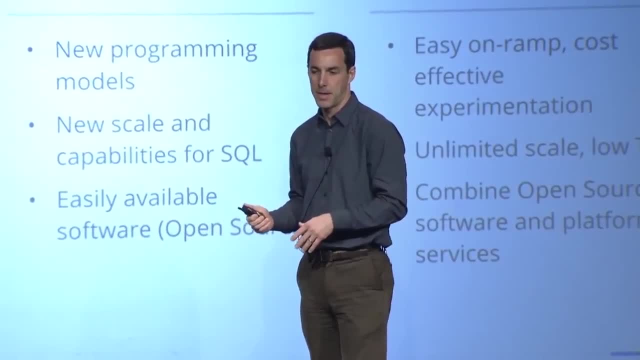 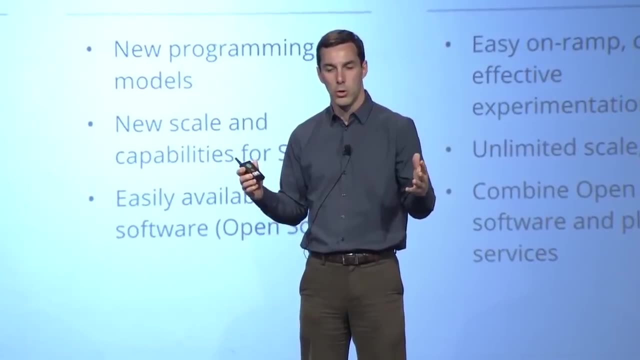 it will remain the cheapest place, the most effective place for big data processing. And finally, the third aspect of the cloud construction law for big data is that on a platform like Google, you have a chance of using a mix of platform-provided services fully hosted. 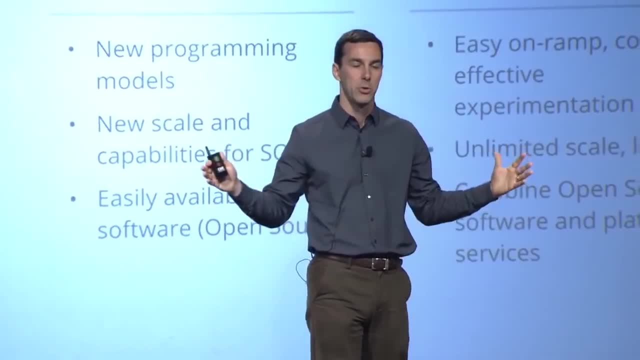 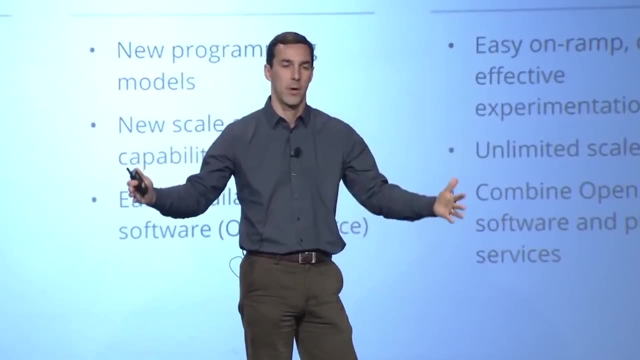 fully managed as well as open source software, And you use them. it's not one or the other, you use them together. they share the same data, they share the same authentication system. It's one environment where you can seamlessly make use of one or 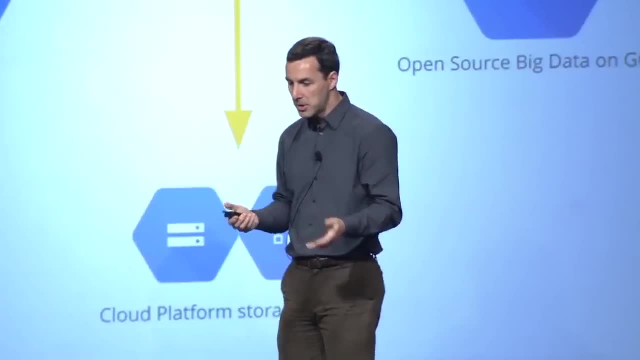 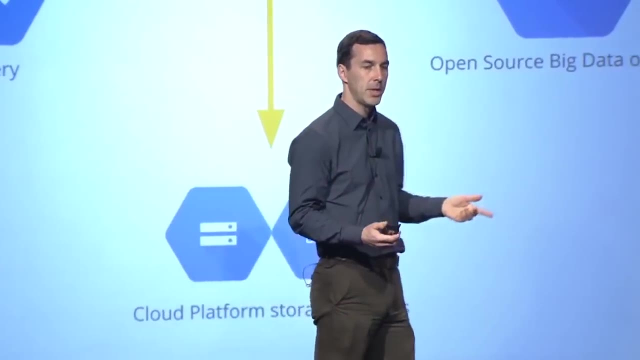 the other, use them together, transition between them, And that's one aspect that we're gonna illustrate today. So we have two sessions on big data. In this session, we'll focus on BigQuery And Jim is going to describe new features, new scalability achievements. 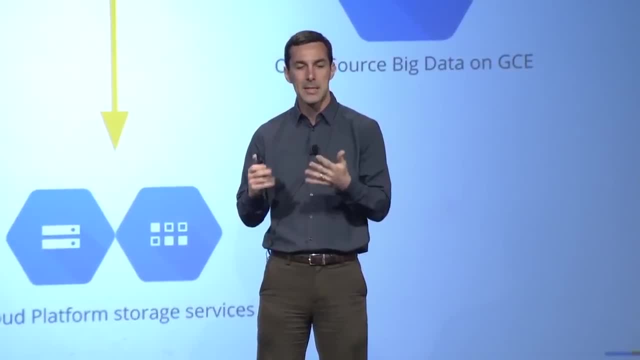 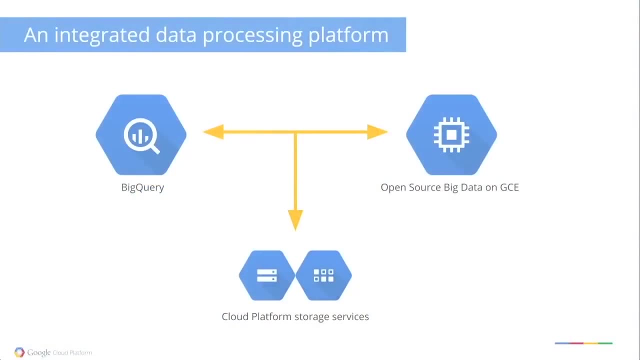 new and more detail about a new pricing model. And as he describes all that, keep in mind everything he's describing. you get that with no installation, no configuration, no monitoring. You just come sign your query, get your result, that's it. 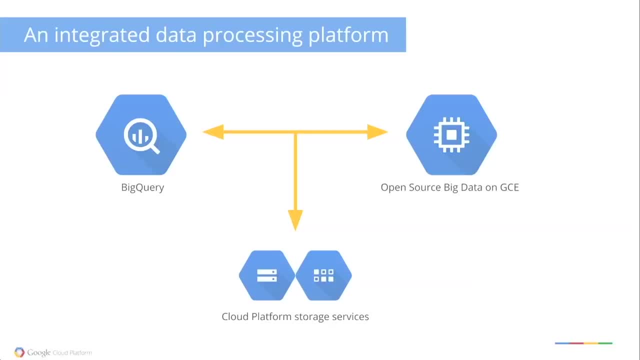 This is the best of a fully hosted, the easiest to use, most productive services. And then at the same time, we'll have, at 3.30, here in the same room, another session all dedicated to running open source big data processing software on Google Cloud Platform. 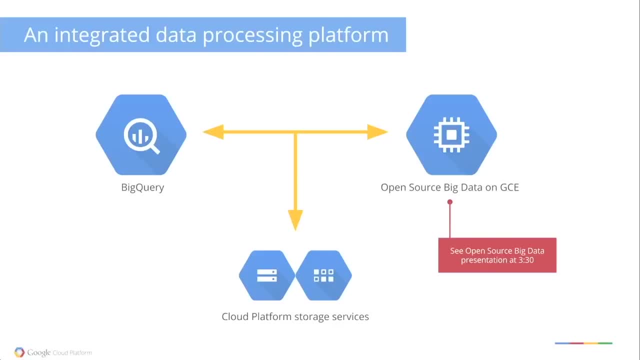 And there we're going to show how the quality of the infrastructure, the compute, the storage, the network, and give you excellent performance And excellent cost performance running open source data software. We'll talk about some of that we've done to implement open source APIs to. 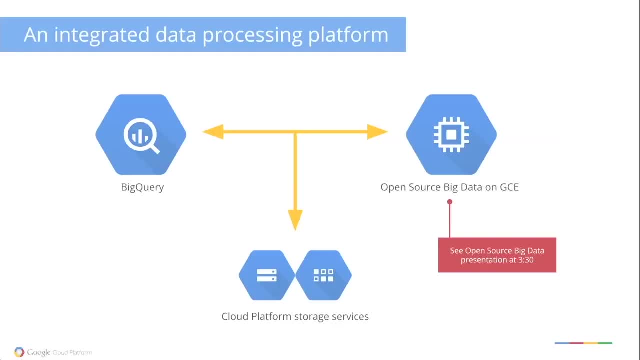 natively connect to other sources. We'll talk about some tooling that we've put in place. We'll describe in detail how much value you can get from running open source software for big data at Google And keep in mind between these two sessions, hopefully you'll be able to. 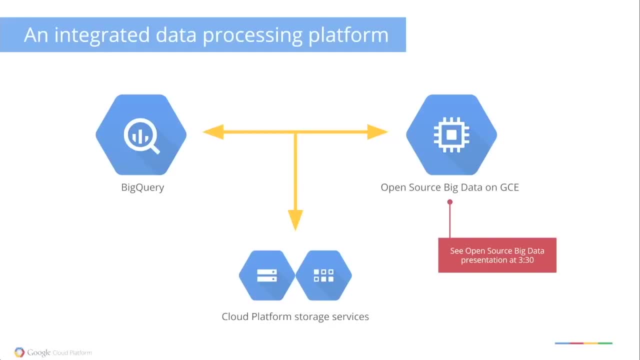 able to attend both. this is really one platform. We've broken that into two sessions, but it's one data set, one environment for you to bring your beta processing. So for now, I'll yield to Jim and he's going to give us all. 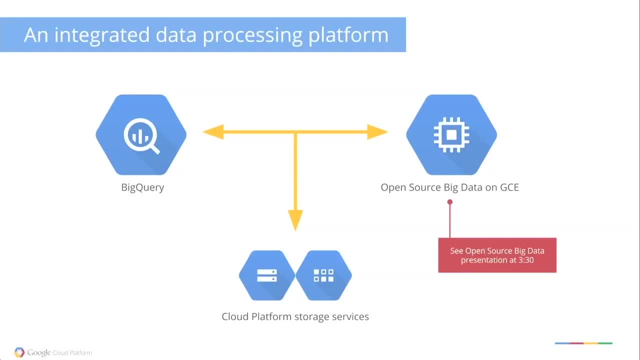 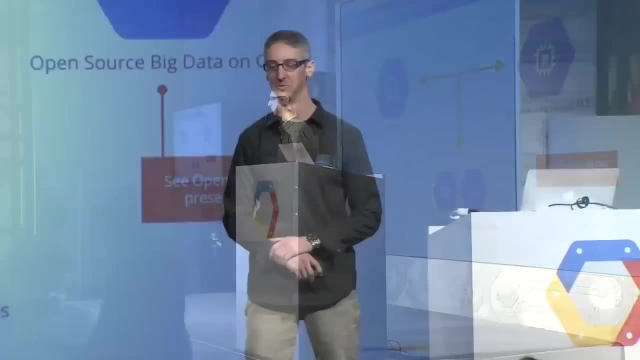 the goodies about BigQuery. JIM LECINSKI- Thanks, Thanks, William, and thanks everybody for coming this morning. I'm really excited to be here to tell you about the latest innovations we've got going on in BigQuery. 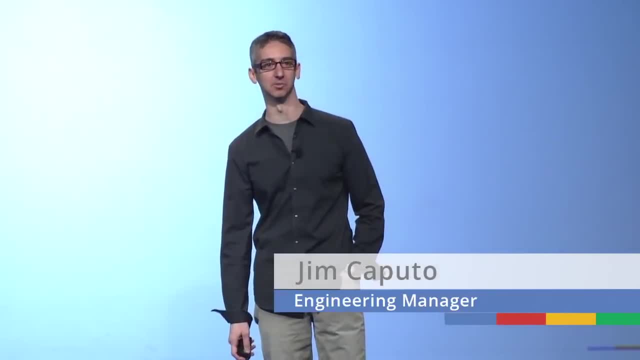 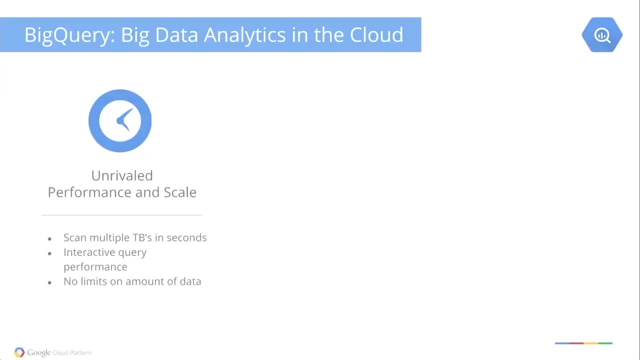 So we launched BigQuery a little under two years ago, May of 2012.. And what we brought to market for the first time was the ability to scan multi-terabyte data sets in just seconds. This capability was previously unheard of. This unlocked a whole new set of use cases: the ability to 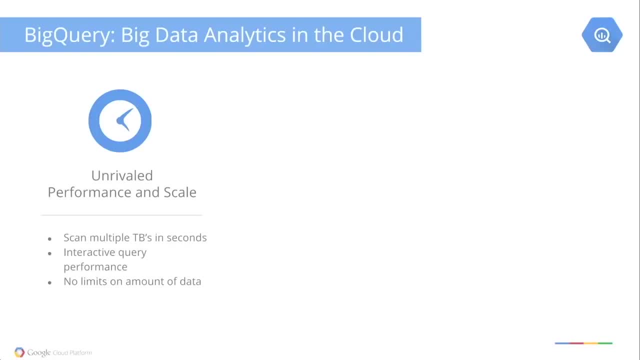 finally do interactive analysis over huge data sets. We combined that with tremendous ease of use: no provisioning, as William was talking about. no figuring out. how many machines do I need to do this? how many cores would it take to process a terabyte of data in seconds? 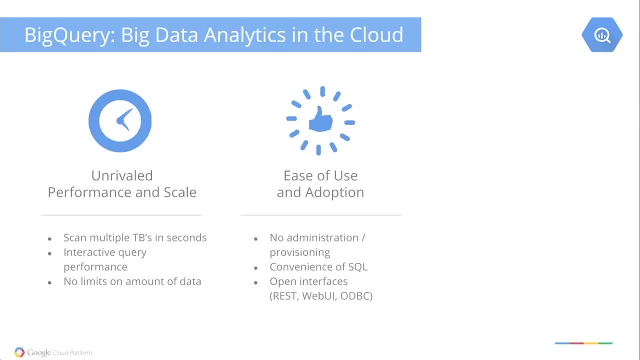 And we make it convenient, right The convenience of SQL and open interfaces like our REST API, web user experience, SQL 92-compatible ODBC driver And, finally, we introduced this notion of big data storage. We wanted to improve the experience around how you 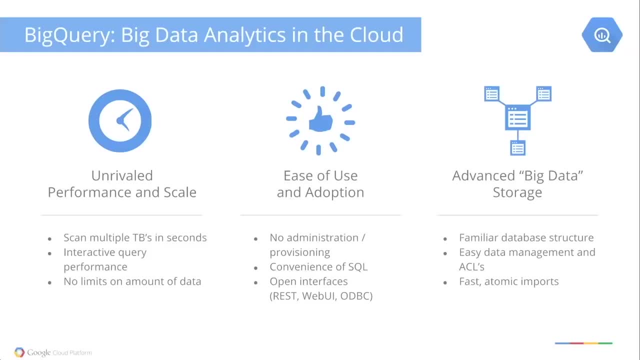 actually interact and manage your data. Most of the large data processing- big data processing- is done on large files, large quantities of files. We felt like a familiar database structure is what people really wanted, though. They wanted easier data management. They wanted to be able to and share their data. 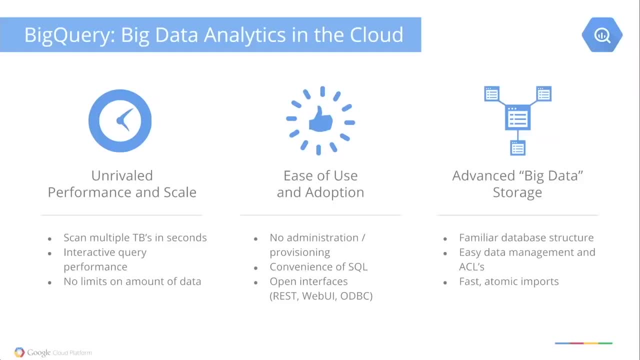 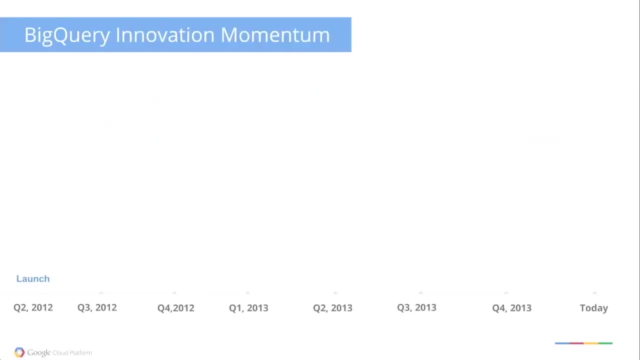 After all, you're moving all this data into the cloud. Shouldn't it be easier to collaborate with your coworkers? right, And we made it easy and fast to get your data into the system. So we've been hard at work over the last two years and 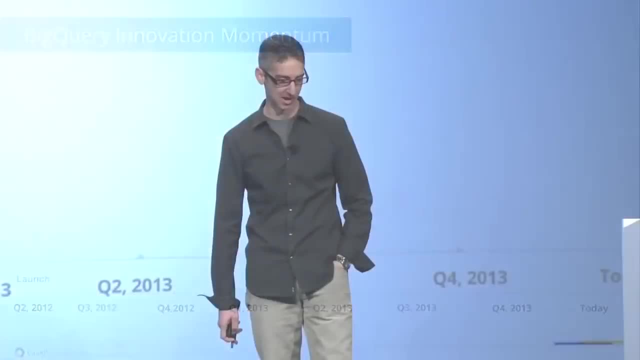 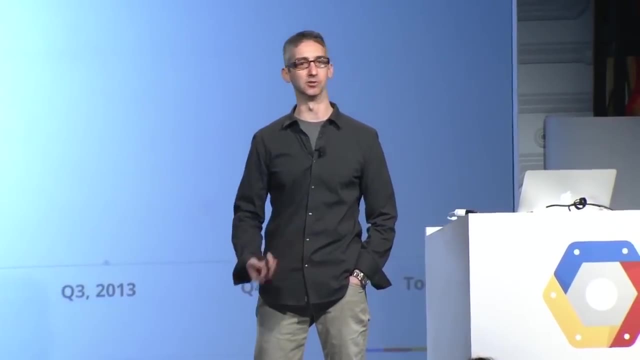 we've added quite a few pieces of new functionality along the way. Shortly after launch, we introduced batch processing, So you had the ability to queue up all of your jobs and then we would just run them when idle resources were available. Clearly, not every use case requires. 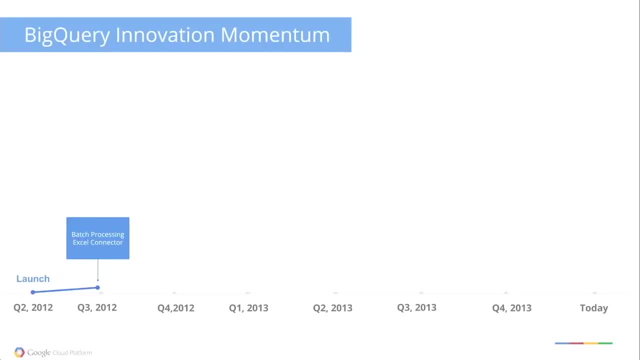 interactive performance. The Excel connector made it easy to use Excel as your primary front end, if you desired, and then use BigQuery as your primary big data back end. I've got a lot more in terms of partners to talk about in a moment. 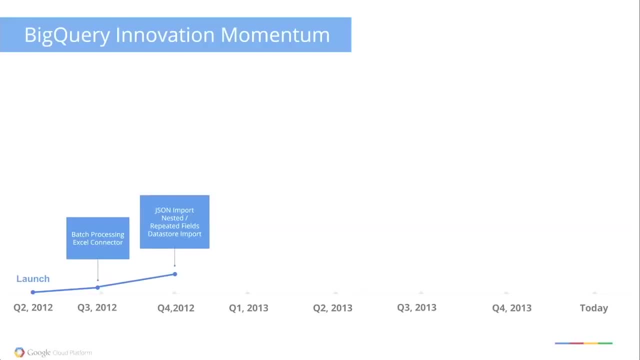 Next we added JSON import in addition to sort of standard CSV imports. JSON's obviously valuable, pretty ubiquitous standard in terms of moving data around but, more importantly, unlocked, nested and repeated fields for us, which is a pretty powerful although admittedly a little bit complex data. 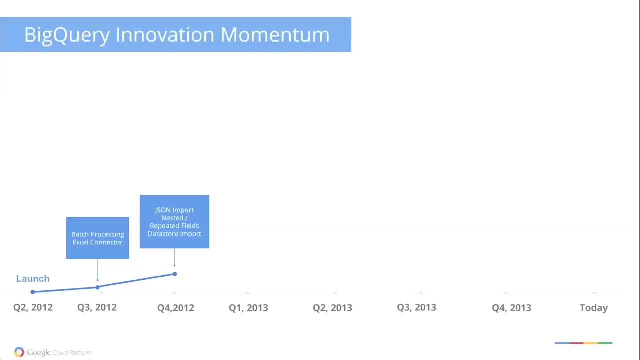 structure to make use of. We also made it possible for us to use JSON as a standard and we're able to bring data stores. If you have a cloud data store instance, you can back that up and then bring it right into BigQuery for analysis. 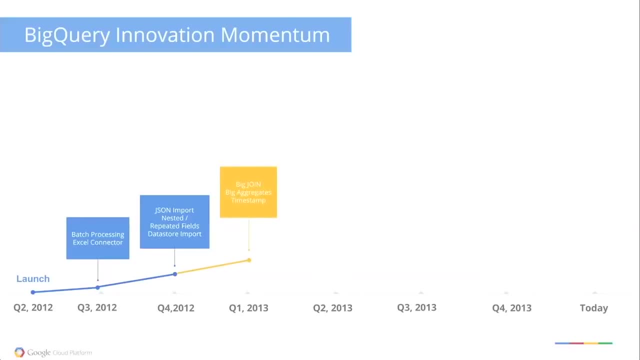 Or, as mentioned earlier the beginning of last year, Big Join: the ability to join two arbitrarily large data sets together, regardless of join key that you're operating on. Big Aggregates the ability to group on something that has potentially millions of distinct values. 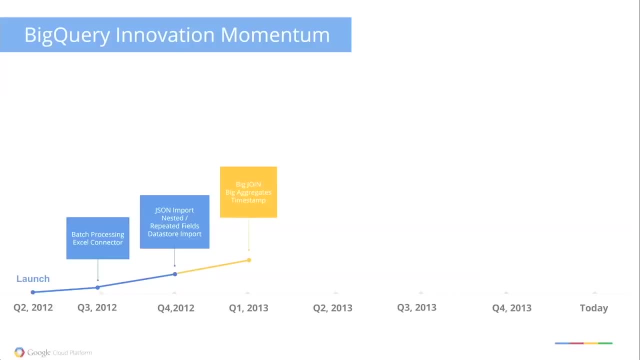 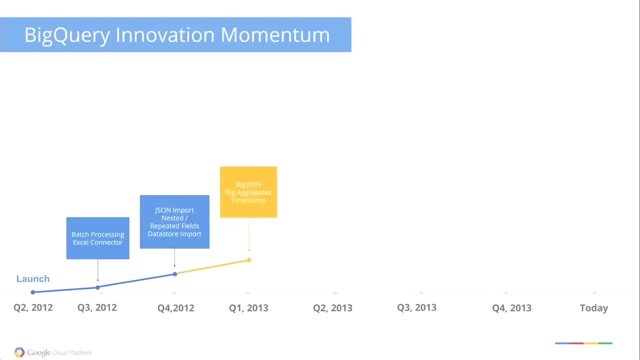 So we're furthering that goal of making this more database-like. The standard timestamp data type and the accompanying functions that would go with that After that large query results. So not only were you able to query data of unlimited size, you can now generate data of unlimited size. 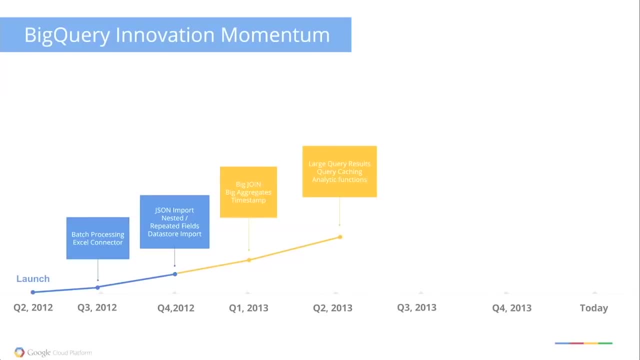 So all of a sudden we started seeing more and more use cases emerging. We started with that interactive analysis. We started seeing people doing more ETL processing, for instance, on top of BigQuery Query caching, just to help out application development. 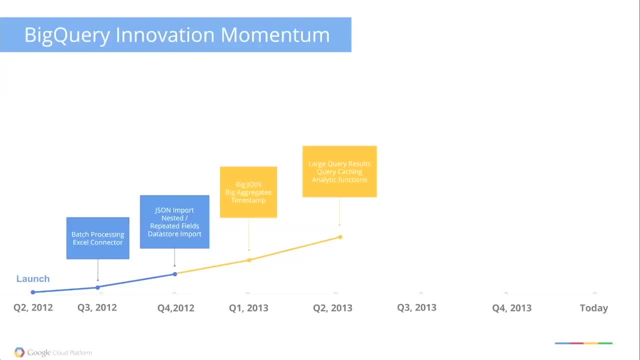 reduce costs, speed things along. Analytic functions: We continue to invest in our SQL engine. Near the end of last year, the streaming API, It actually launched with 100 rows per second, initially combined with that feature. you saw that Eric demonstrated with table decorators. 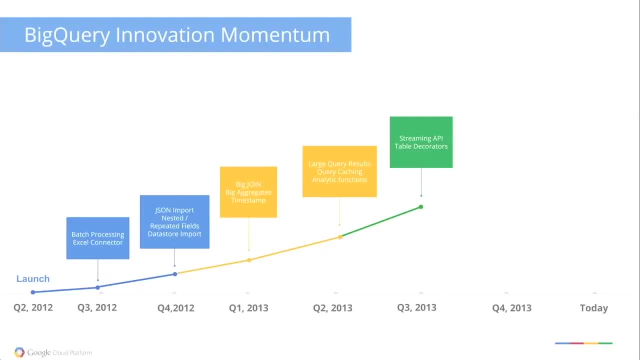 So the ability to just slice into- I only want to see the last two hours of data. for instance, At the end of last year, Google Analytics integration- I'll talk more about this in a moment- And finally, today, a bunch of new features coming out. 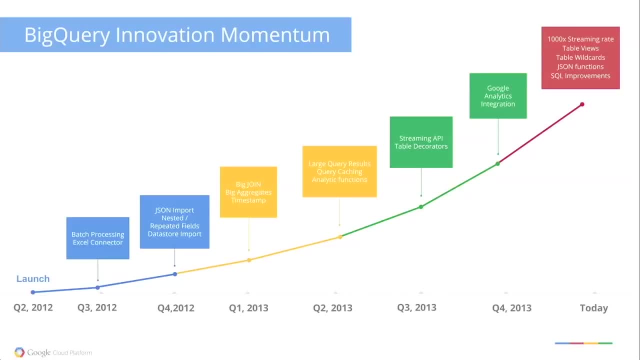 We've dramatically increased the streaming rate, as Eric showed you, Up to 100,000 rows per table, now Table views, Again, extending on that goal of advanced big data storage. We want this easy to use. We want you to be able to reuse this stuff. 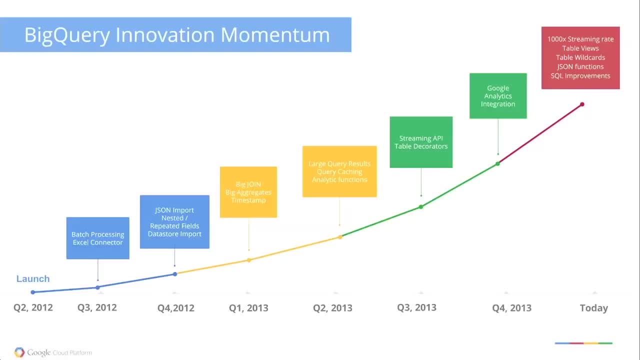 and share large queries across your organization more easily- Table wildcards, So also mentioned this morning the ability to very easily shard your data across many tables. We want to make that easy to use from a query perspective. So, for instance, if you've chosen 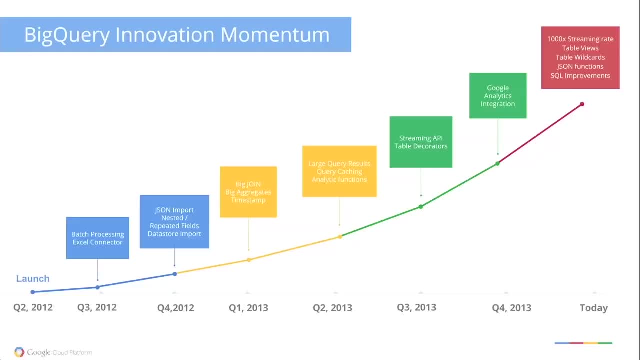 to shard your data across days. you may want to use a wildcard that says: give me that table and here's the date range I want to apply. It automatically just works for you. JSON functions. So if you've loaded up a bunch of JSON in a given field, 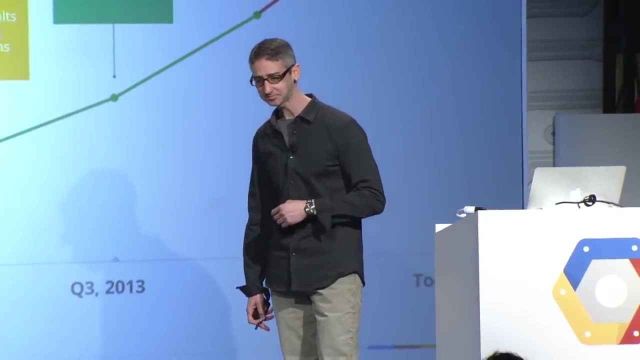 you can use a JSON function to extract out values automatically And finally, a whole bunch of other SQL improvements trying to make us much more closely aligned with the standard SQL 92 spec, as well as a whole bunch of additional improvements, like some of those analytical functions. 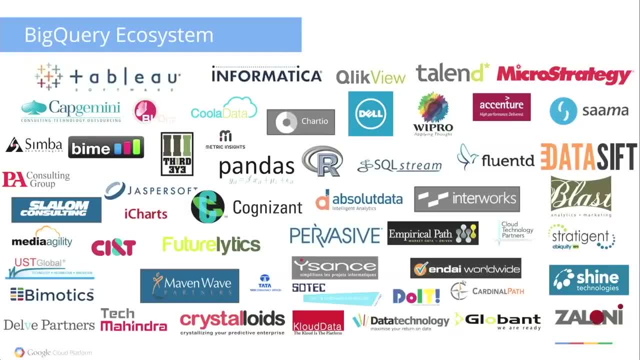 So it's not just us. The ecosystem around us has been going at incredible speed. We've really been impressed by this. We've got a great partnership, for instance, with Tableau. We've spent quite a bit of time working on the technical integration there. 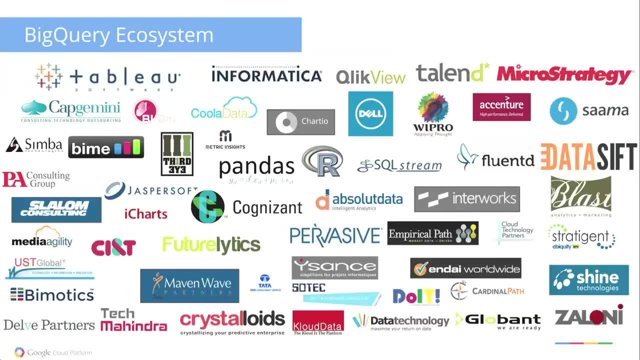 We've been able to see whole new use cases emerging in that space as well, actually bringing interactive performance to a visualization and data analysis tool like that. It's been tremendous. I saw a great example of Pandas, so Python and analytical functions done there in the open source community. 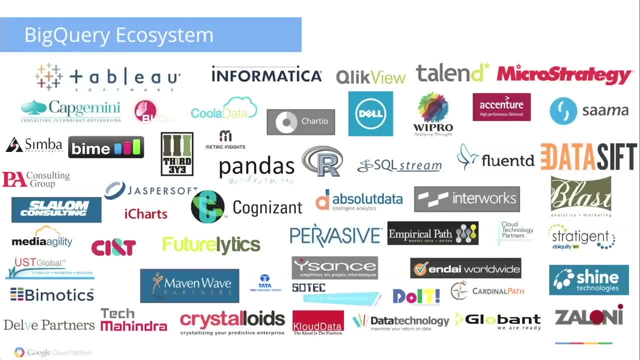 As you can see, a whole bunch of other providers all working around us. So thanks for all your efforts out in the open source and partner community. We're sort of excited to see where this can go next, building on top of the BigQuery. 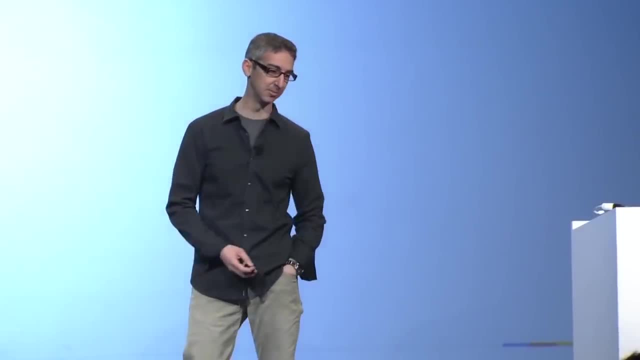 We're excited to see where this can go. next building on top of the BigQuery platform. So BigQuery streaming. Let's dive into this a little bit further. As demoed this morning, we can do 100,000 rows per table. 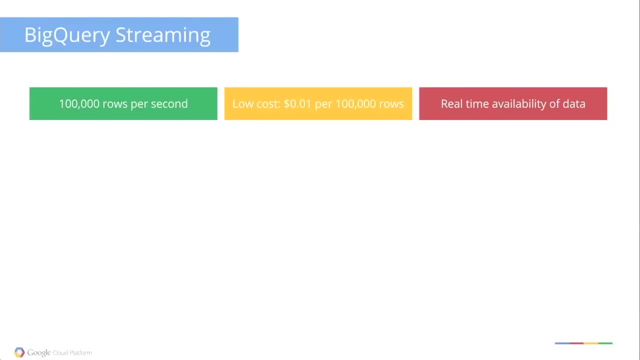 at a low cost of just one penny per 100,000 rows and real-time availability of that data. This dramatically simplifies the amount of infrastructure that you have to build and maintain on your side. No longer do you need to batch up records. 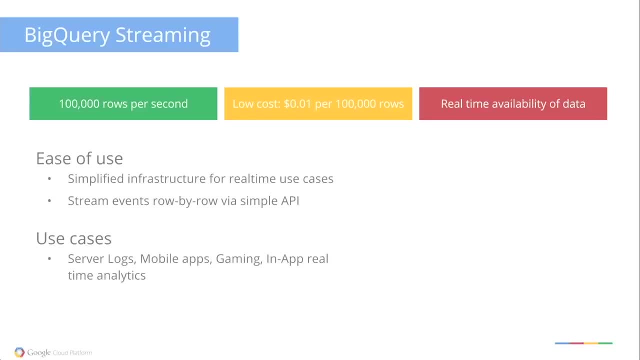 and figure out when you want to submit those and what latency or frequency they're going to come into the system. And the use cases are endless here. So for starters, For starters, you can see an example like that distributed application that Eric built. 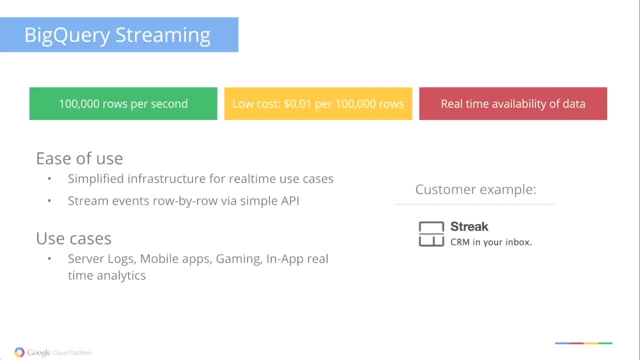 But we're starting to see other examples emerging And working with a customer Streak, one of our early adopters. they were impressed by this. They were able to use streaming to reduce the amount of infrastructure, of course, to simplify the infrastructure to bring. 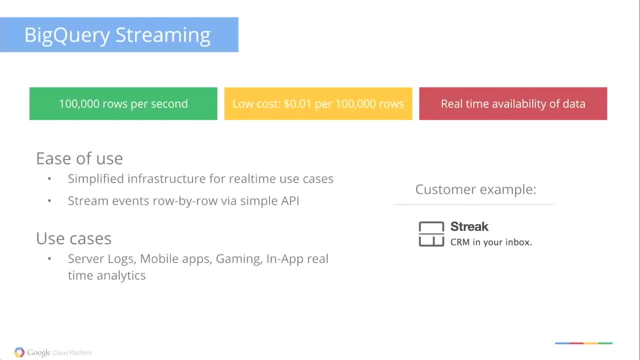 their data into the system And so great they were able to continue using their standard reporting. What they found were new use cases emerging All of a sudden. they had user support scenarios that would come in And rather than have to go to one system and to figure 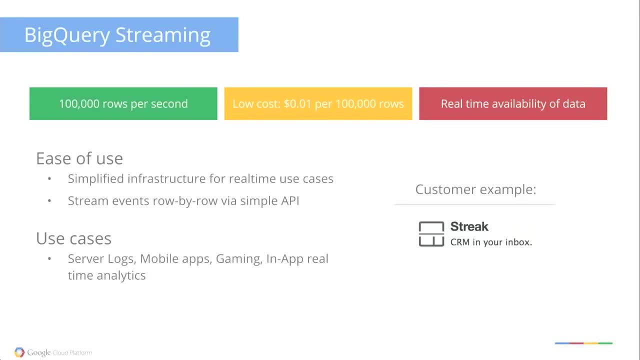 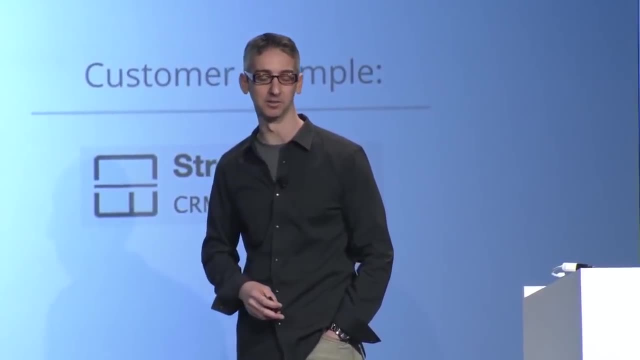 out the debug logs. they could go to a single system. look at the debug logs right alongside. what was the historical behavior for this customer? What was their user experience over the last month or so? So we think this is the best of both worlds. 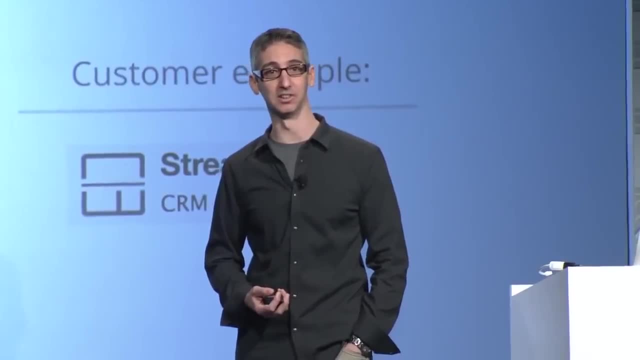 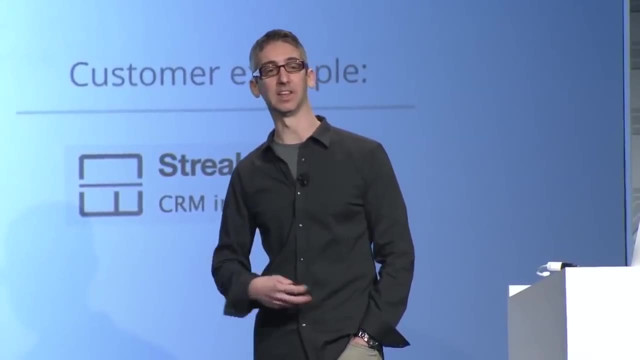 It gives you the flexibility to do that real time processing that you desire when you need it, that low latency processing, while also bringing that data into a storage system that's capable of doing your full historical analysis. So there's nothing disjoint here. Everything is all done in one location. 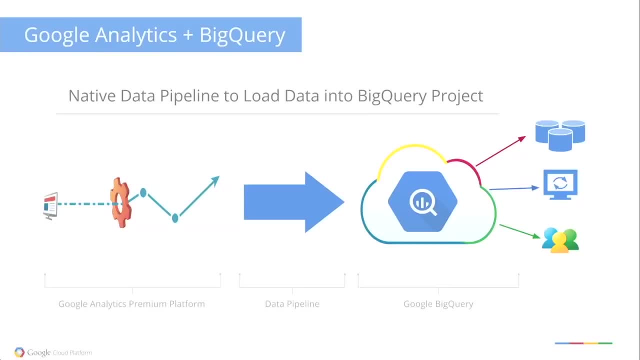 Moving on next, I'd like to deep dive, for sure, into Google Analytics. For the first time, Google Analytics customers are now capable of bringing in completely unsampled, row by row, detail of their analytics data. This was previously unavailable, And the volume of data here is tremendous. 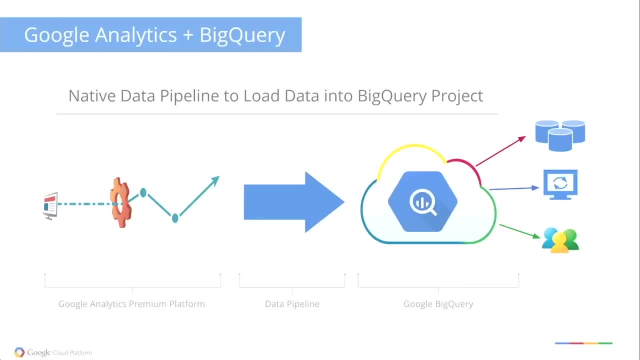 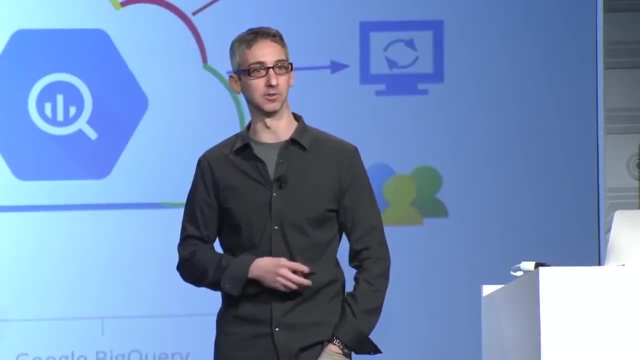 Bringing this data into the system is done completely for you, automatically, via a managed pipeline behind the scenes. Bringing this data in couldn't be any easier for you. All you need to do is sign up for Google Analytics Premium. The data automatically arrives on a daily basis. 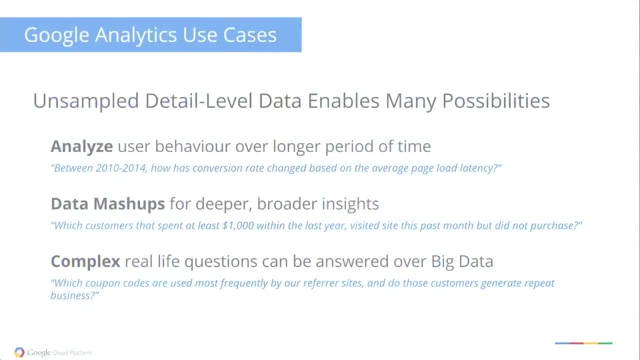 So we've already seen quick adoption here. The number of use cases are essentially endless. In talking with some of our early customers and website owners, the first thing they were amazed by is the volume of data that they could actually analyze inside of BigQuery. 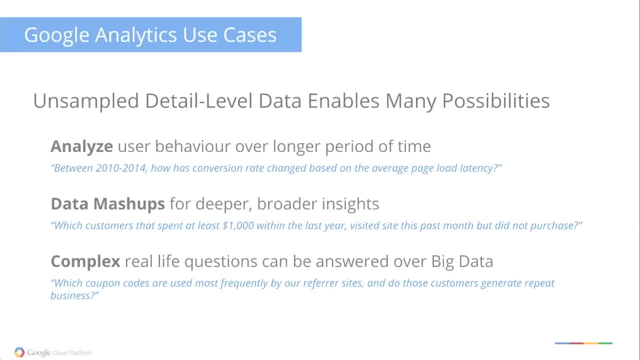 No longer were they looking at month over month changes. They were looking at year over year changes over many years, something just previously they couldn't actually endeavor to do. Secondarily, we've seen quickly customers are actually uploading their transactional information, which is pretty exciting. 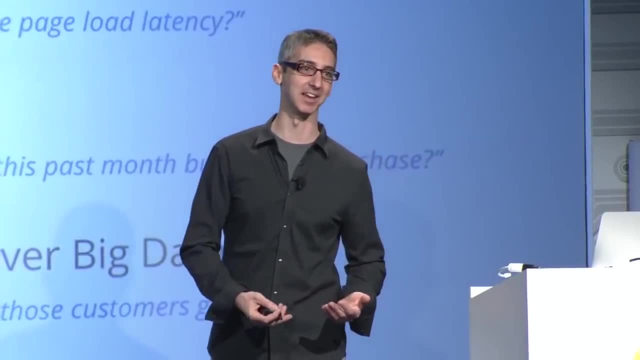 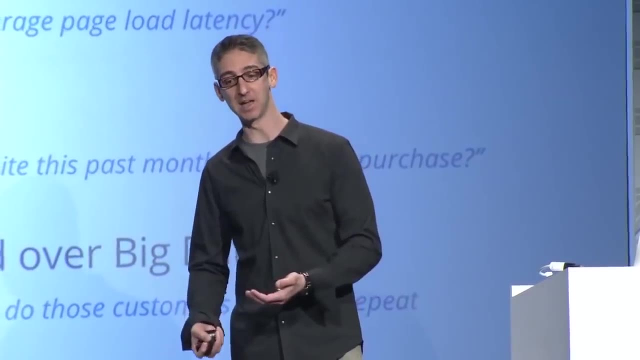 because now they can do those big joins, those data mashups They can actually look at. in this case, the customer is interested in trying to figure out. why are some users spending a fair amount of money on their site? They come back, but they're not repeating their purchases. 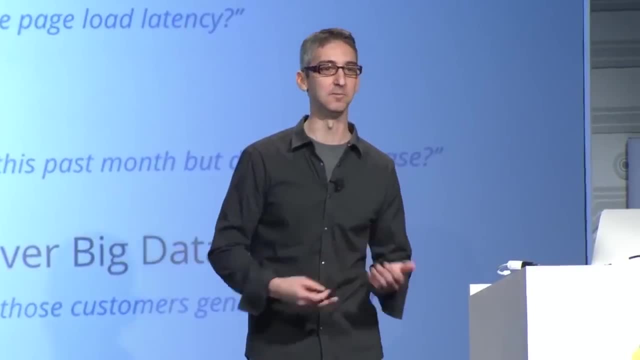 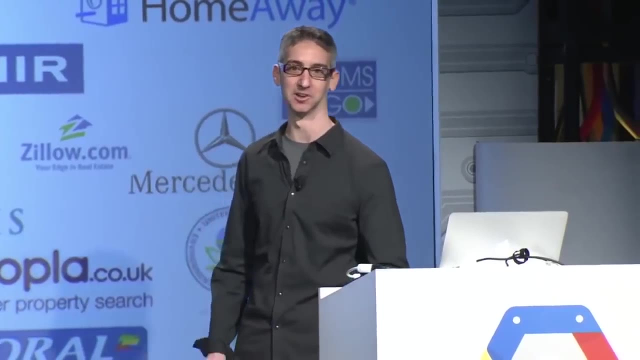 What changed? And then there's another example as well. So the value here is incredibly high. We've seen tremendous adoption In just a few months. a whole bunch of huge customers have been coming online Huge, Huge data volumes and interesting use cases. 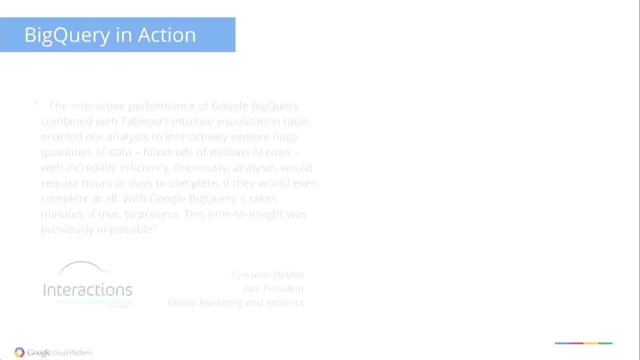 So I wanted to look at a few other use cases I found interesting Interactions Marketing. Interactions does on-site retail marketing, So they're actually out at storefronts doing marketing campaigns. So actually maybe a sample of some sort that they're distributing. 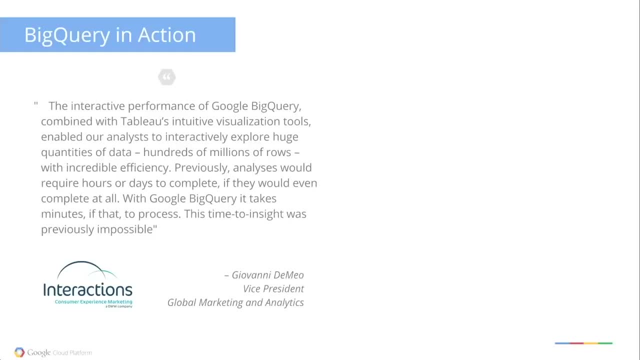 And they wanted to understand the answer to what I thought was a pretty straightforward question. They wanted to understand what's the impact of weather and weather on these retail marketing campaigns. As it turns out, their analysts had struggled to do this for quite some time. 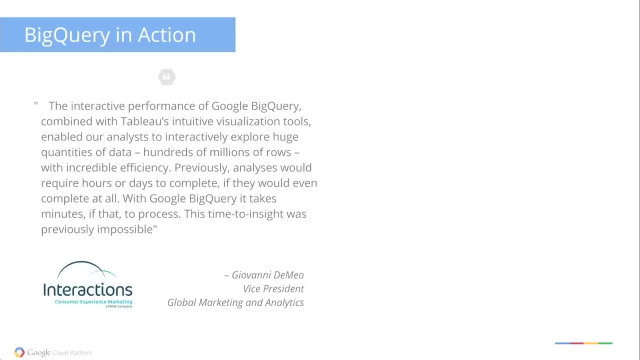 The data volumes were just too large. They couldn't perform that data mashup. But I love this quote here from Giovanni. He says analyses would require hours or days to complete. With Google it took just minutes This time to insight was previously impossible. 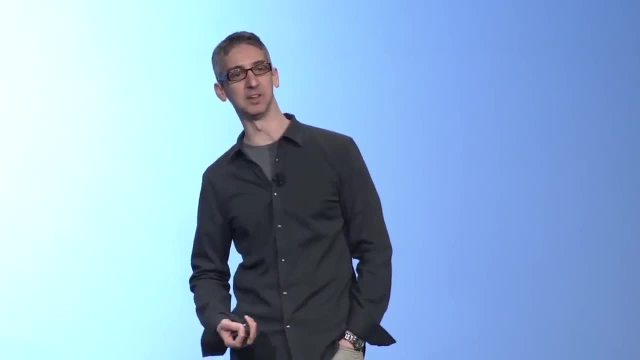 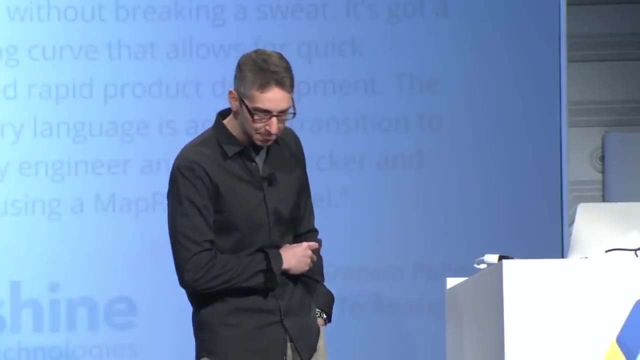 So using the power of Tableau as their front end and BigQuery as their big data back end, deriving insights that were previously not possible to generate In the past. This next one came from Shine Technologies. I was really interested to learn more about this. 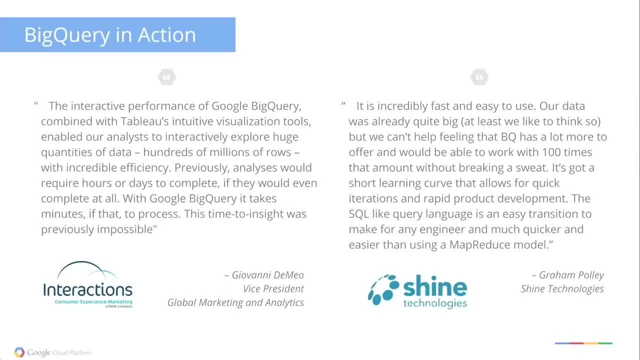 In fact, they're here today, So I'm excited to have them in the audience here. So Graham actually posted a tweet a couple of months ago and said: hey, we've been really successful with this BigQuery product. What it turned out was they were actually. 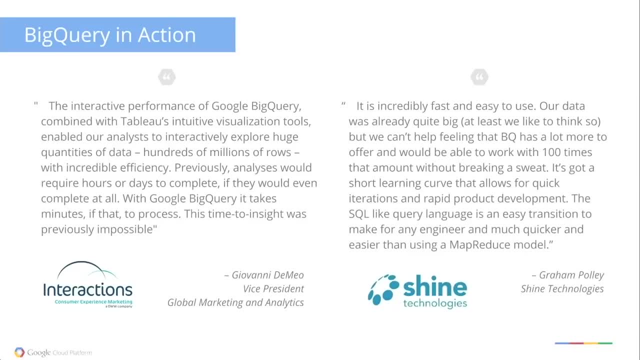 struggling in the past to do the data analysis they needed to do on running on just a small sample of the data set that they had in question. They're using ad serving logs, a huge number of impressions and counts that they were trying to push through the system. 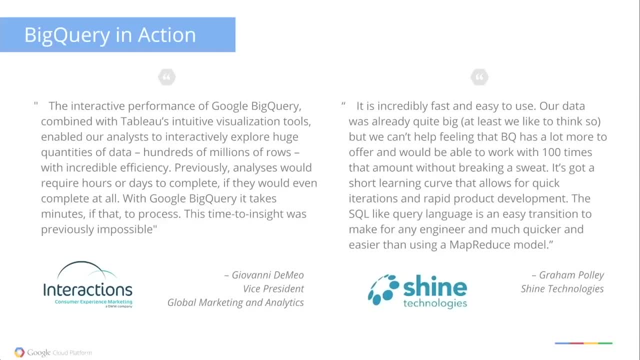 And they were amazed. in a two hour proof of concept effort They went from getting the data loaded to immediately being able to answer questions that were previously impossible. I love the last line here. It says the SQL-like query language is an easy transition to make for any engineer. 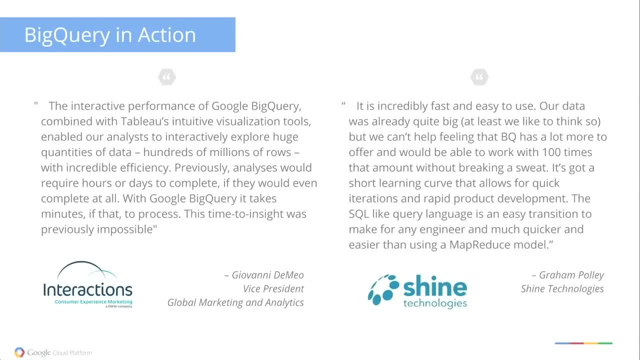 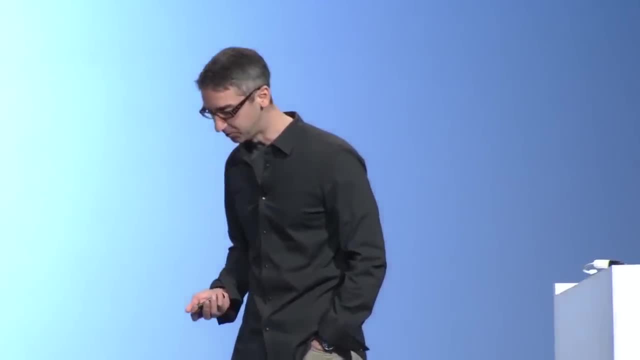 and much quicker and easier than using a map-reduced model. Again, simplicity along with scale. We're trying to drive both of these at the same time. So I mentioned we started with this. It was arguably relatively narrow offering. It was high performance, really fast. 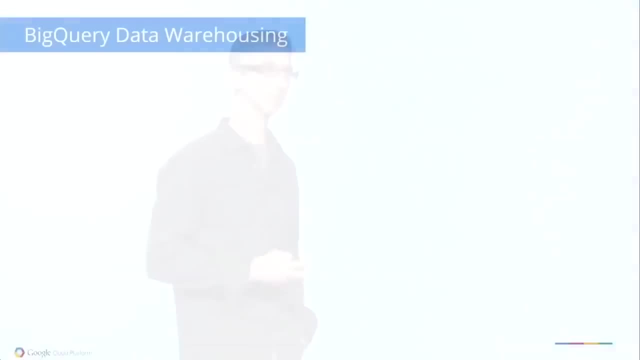 But it wasn't really intended to solve for something as big as data warehousing. Well, that's definitely changed over the last two years. Our friends over at Motorola have made huge use of the system and are using it as their primary data warehouse for some of their most important data. 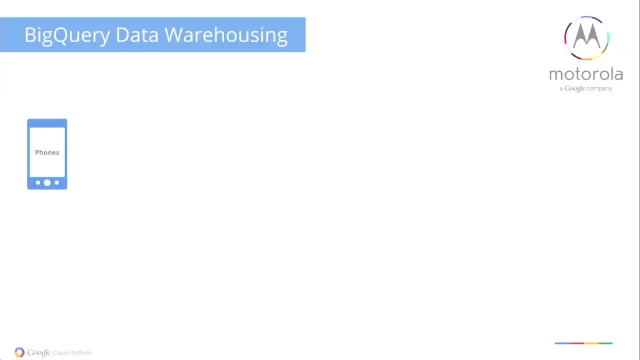 So to walk through this, their most important data is their telemetry data that they're collecting off all of their devices out there- Obviously hundreds of millions of Motorola phones. They ship this data. It's up through App Engine multiple times per day. 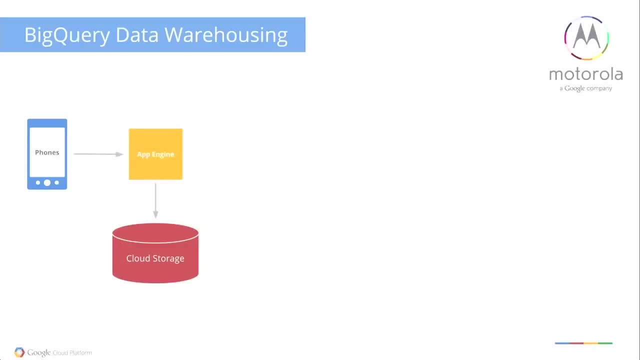 App Engine does some lightweight pre-processing and then drops it into cloud storage for archival purposes, which is fine, but it's not particularly actionable sitting there. Instead, as quickly as possible, move that data over to BigQuery storage, where they can begin to take action on it. 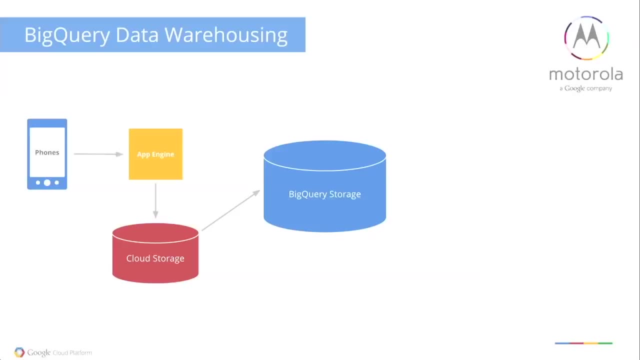 Motorola was running the majority of their data processing in-house. previously They had a rather large Hadoop instance on their own private cluster And they came to us less than a year ago and really started investing in the cloud platform. As it turns out, they went from basically zero bytes. 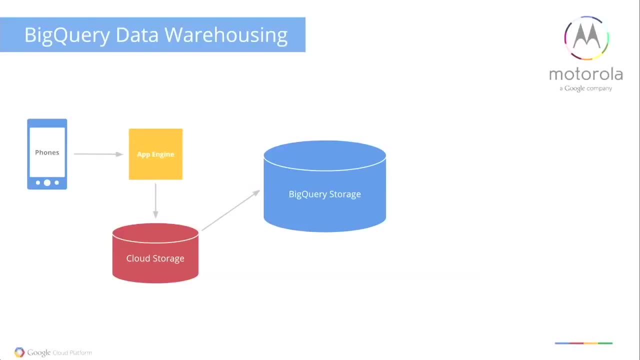 in BigQuery a little over a year ago to now having many petabytes of data in storage, And they actually are still using those same Hadoop Map Reduces. So they're running those Map Reduces now on top of the logs that have been brought into BigQuery. 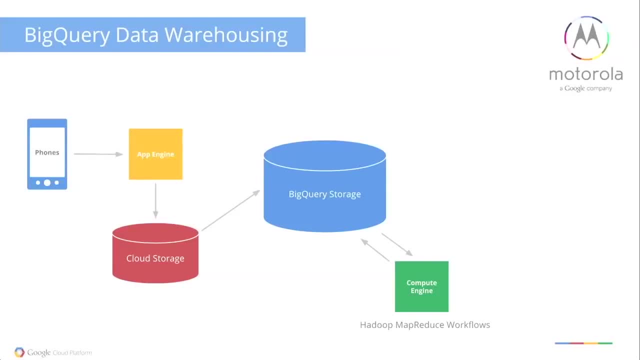 storage and generating the downstream tables they need for analysts to consume. On top of that, we've seen them actually migrating a decent number of their workflows over to BigQuery. So Map Reduce is great in some instances. SQL solves for other cases. Might be simpler to use in some circumstances. 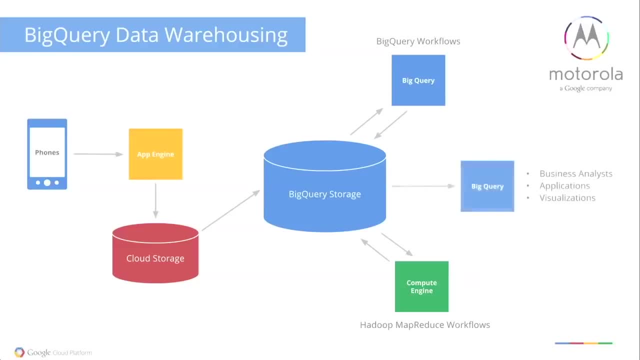 And then finally, once that data is all processed and ready for use, it's moved downstream in general for all of their analysts to take advantage of Hundreds of analysts around the company running queries all day long: building applications, visualizations, dashboards. 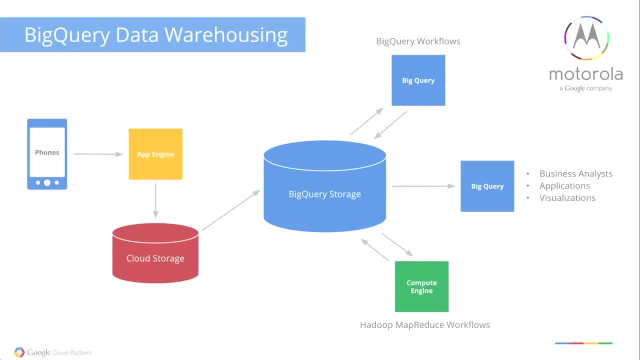 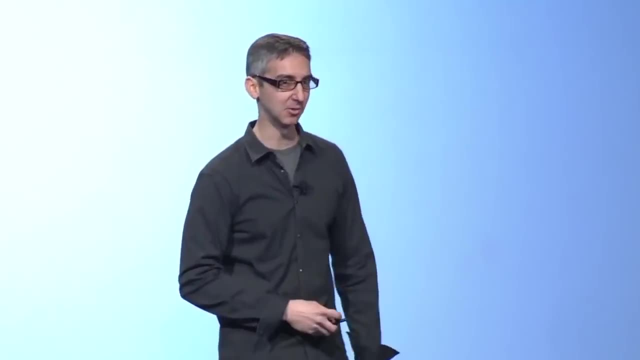 So, whereas previously we assumed that BigQuery was primarily intended as an analytics engine, now we're seeing it expanding, seeing it going into this data warehousing role. So I've harped on this quite a bit. now, BigQuery storage, It's more than just data warehousing. 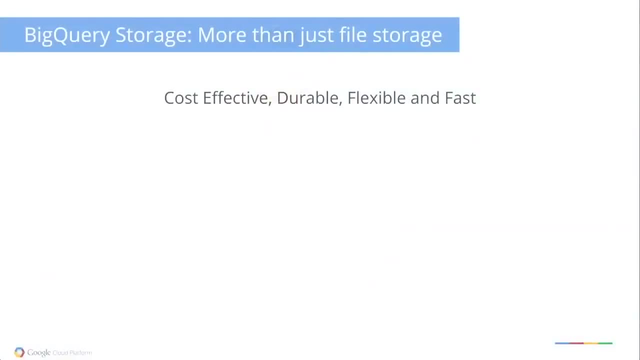 It's more than just file storage. We've invested in it quite a bit and we continue to make improvements. It's, of course, everything you would expect from cloud-based storage, right? It's highly available, highly durable. It uses an optimized columnar format underneath something. 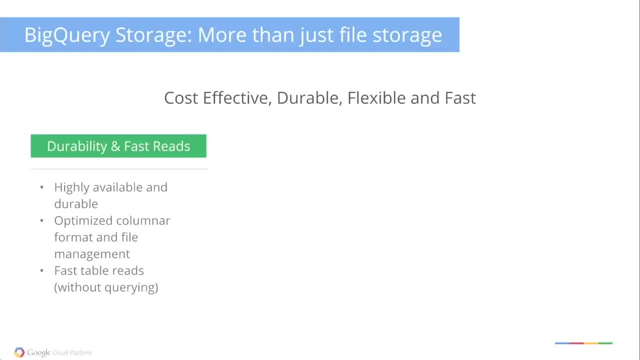 we've built proprietary inside Google specifically for this kind of workload And we take those files that have been imported and we actually do quite a bit of management on top of those for you on your behalf. So, for instance, if you have happened to import a whole, 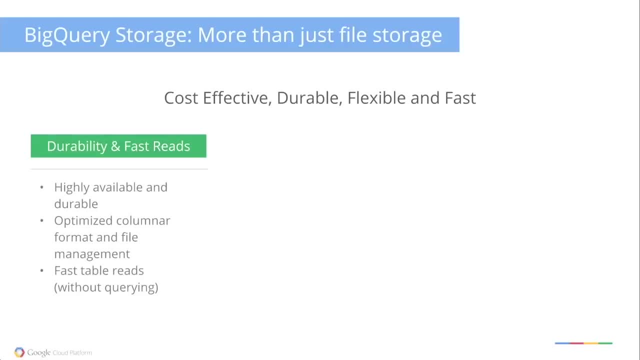 bunch of small files. we'll actually automatically coalesce those over time to ensure that we get the highest possible query throughput, And we offer fast table reads, the ability to read data out of that storage layer without running a query. It's rich metadata, as I said, a familiar database-like. 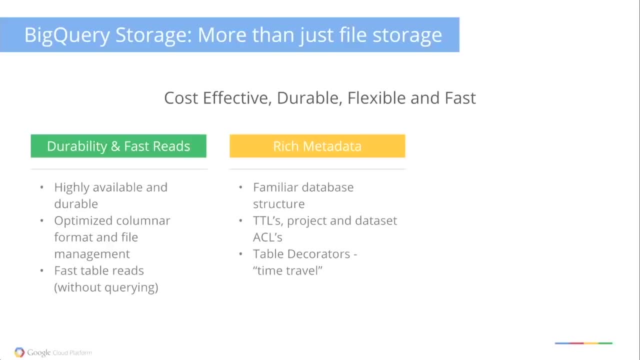 structure, data sets, tables, full fields and schemas, as well as descriptions. we just added in this latest release for each one of those A time to live on tables. Maybe you only want to store 90 days worth of data? You can just expire tables after 90 days. 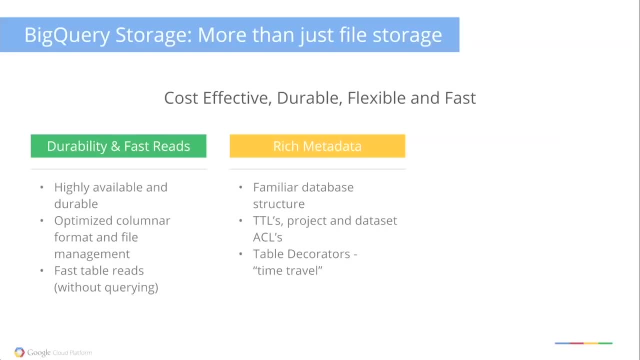 Project and data set level ACLs, so very fine-grained controls. And table decorators. maybe another interesting use case with table decorators to highlight: Imagine: over the last two days you discover that your imports were bringing in corrupted data. You could actually reference the table as it was two days. 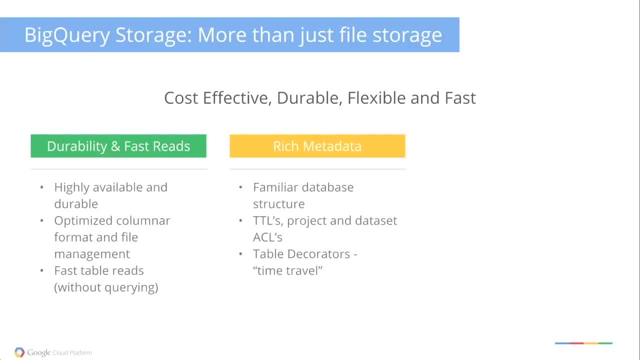 ago. make a copy of it, rerun the imports with your corrected data and off you go- Very easy to interact with. And finally, data imports. We've invested heavily in the standard high-frequency bulk imports. We've obviously got this new improvement now with streaming. 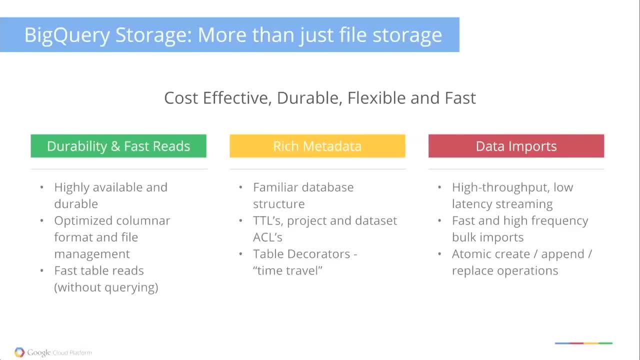 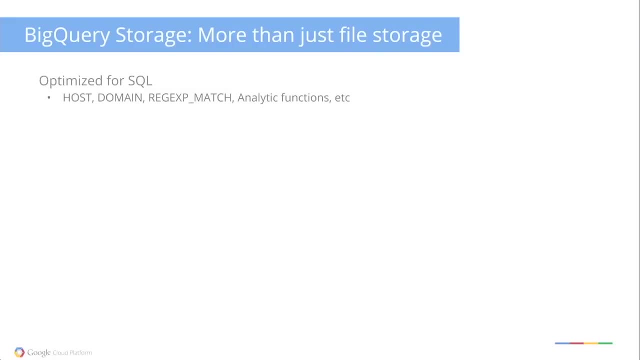 API and we couldn't make it any easier with respect to, again, data feeds like Google Analytics. So BigQuery storage. It's, of course, optimized for SQL. That's the primary interface that we've exposed to you all, And we continue to make investments. 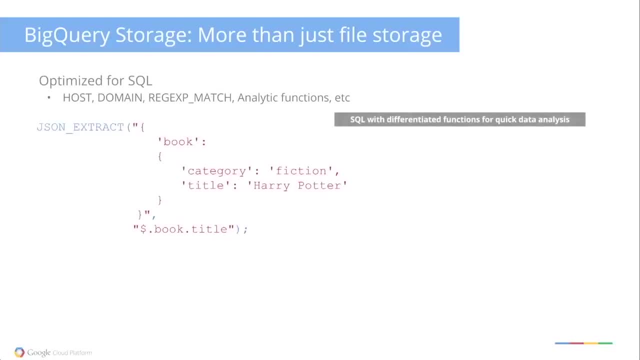 in terms of new functions. JSON extract is an interesting example here, So this might open up a whole new set of use cases. You have your JSON data somewhere. You just bring it directly into BigQuery. You can preprocess it and then generate downstream tables. 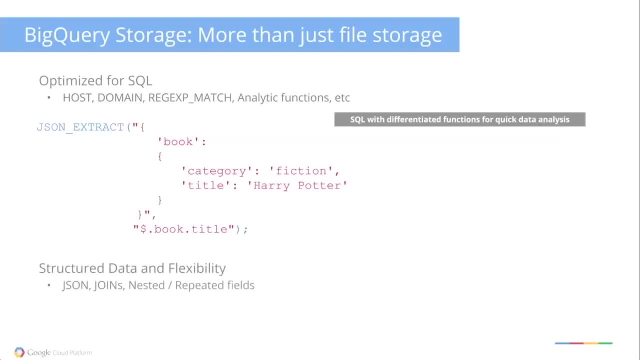 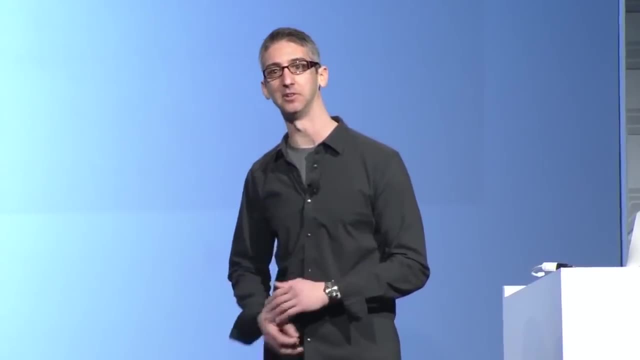 that you want to run your analytics on. So it's a structured data repository, but a very flexible one. With this JSON processing you can add a lot of value to the data right there. You can do these large arbitrary joins And you have nested and repeated fields. 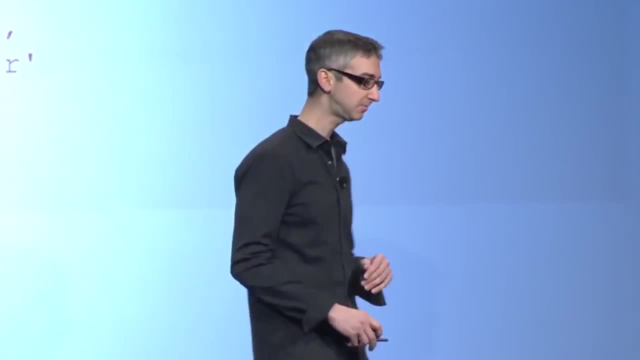 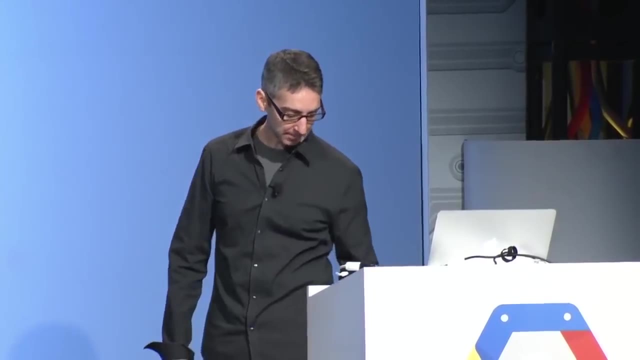 Complex, as I said earlier, but very powerful. So let's take a closer look at that. I'm going to use the analytics data here to look at nested and repeated fields. So analytics applies quite a bit of business logic to all of the hits that are uploaded throughout the day. 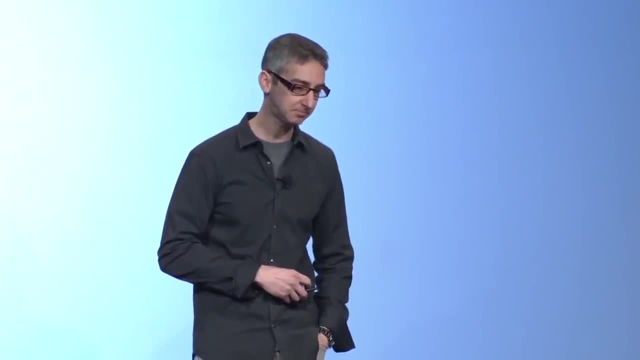 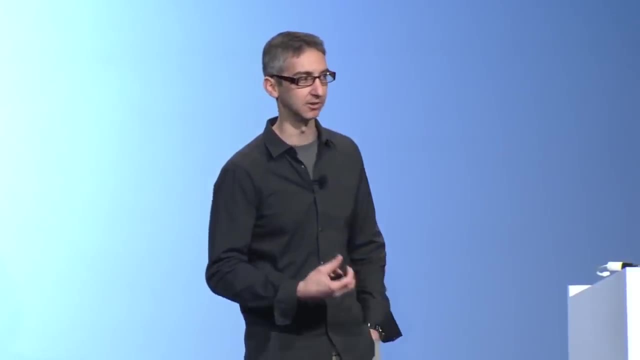 It's collecting every single hit, of course, that somebody has on a given website, With the general goal being they want to generate this, no, this notion of a visit or a session. So all of these hits encapsulated for a given visitor. that's arrived at the system. 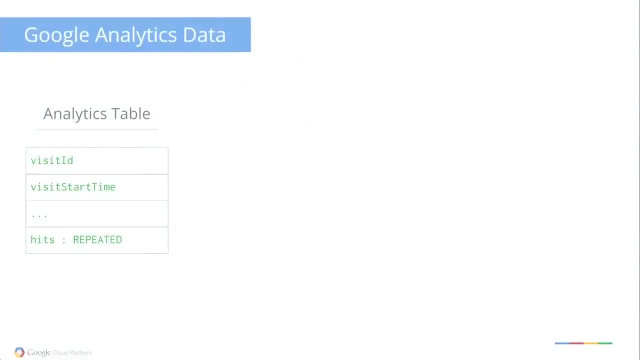 So their schema looks something like this: They have, at the top level of a row or a record, this notion of a visit ID and a visit start time and a couple of other fields, And then embedded within that an array of hits And within each one of those is a hits time. 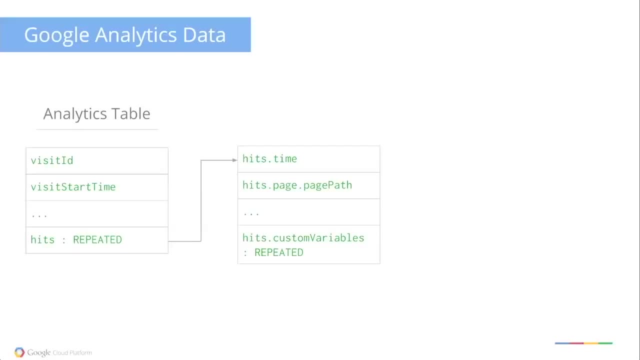 so the offset from the start time And the path, the actual URL that they hit, and a whole bunch of other fields as well. And then just I thought I'd note here yet another repeated field embedded in there for custom variables, if the website owner set those up. 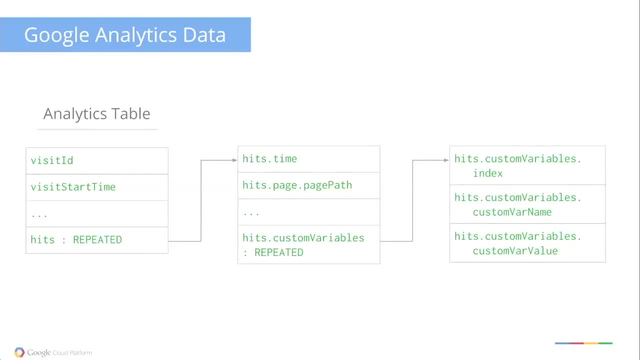 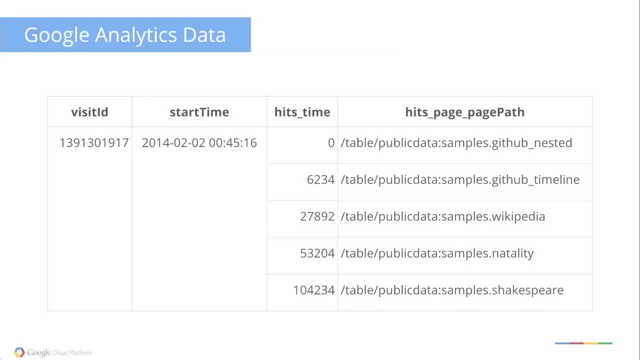 And those would hang off of the- excuse me, the hits array. So what does this actually look like here? So we actually run Google Analytics right on top of that BigQuery user experience that you're able to use. So I pulled out a single visit here from early February. 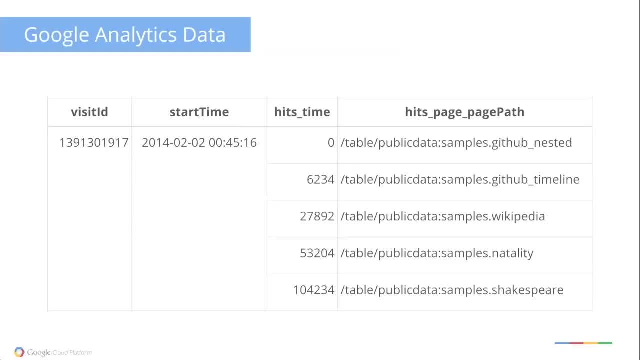 Looking at a few here. I noticed the user went from GitHub, nested one of our public data samples And then moved to the timeline version of that And then kind of proceeded around to the various different tables there, So they were sort of exploring clearly. 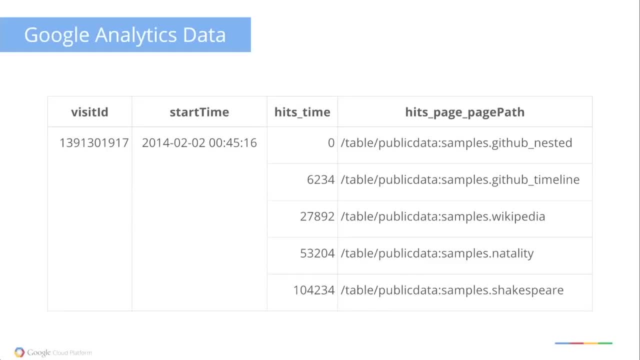 and trying to get a sense of what are those different tables, what can they do with those? So I started thinking about an interesting use case. I was kind of wondering how many people have done this same thing Or how many people have transitioned, for instance. 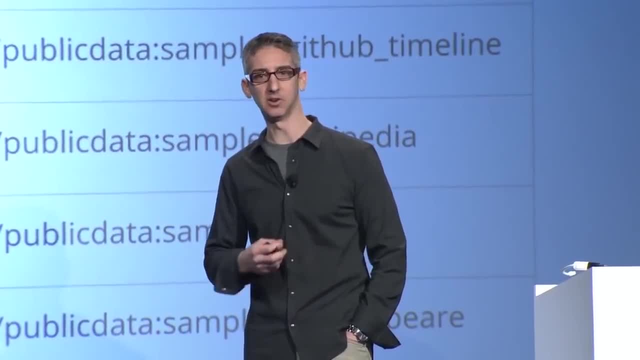 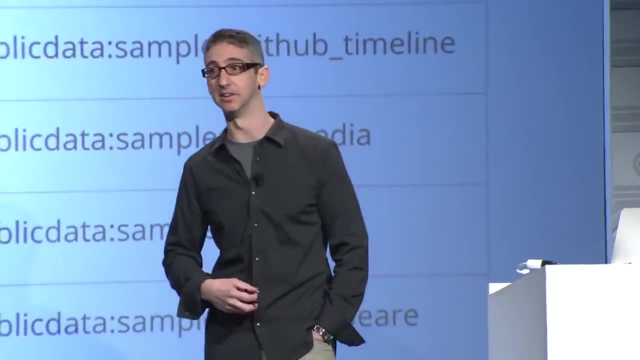 from GitHub nested to GitHub timeline. How would I go about solving that question? And maybe that's a bit contrived, but you can imagine this- in a given e-commerce site, maybe a travel website. You're looking at a hotel details page. 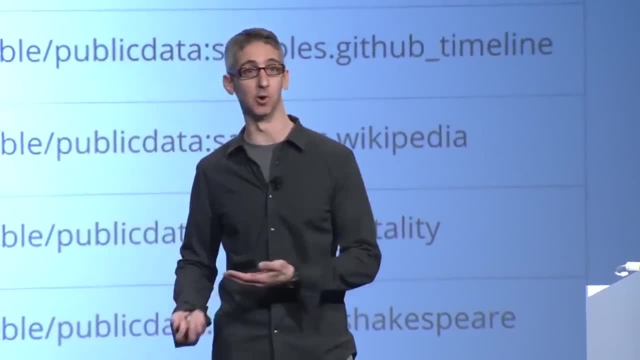 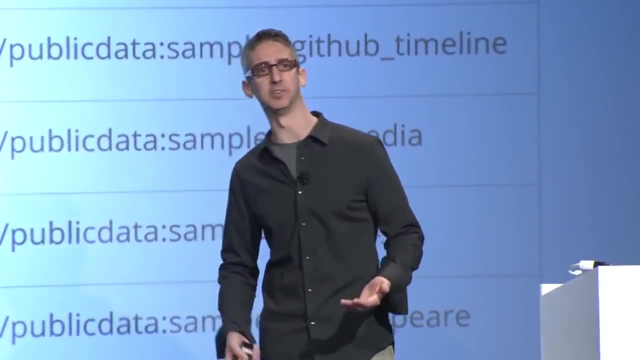 And you wanna see how long does it take for people to transition from the details page Over to the purchase page. Okay, that might be a little more interesting in that scenario. Maybe something's changed, or maybe it varies by region or by hotel. 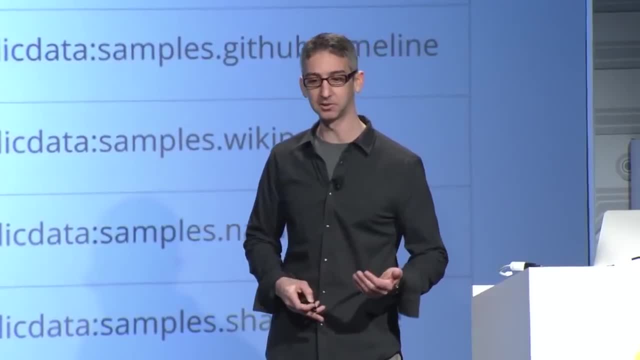 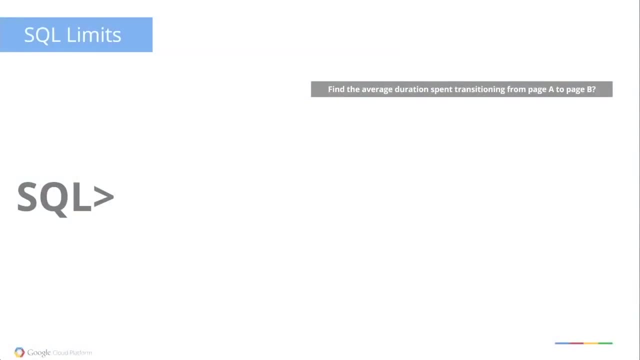 And maybe you need to change your marketing on those pages. So I set out to write this. I wanted to find the average duration spent transitioning from page A to page B, in this case those two GitHub tables And, as it turns out, the sequel for. 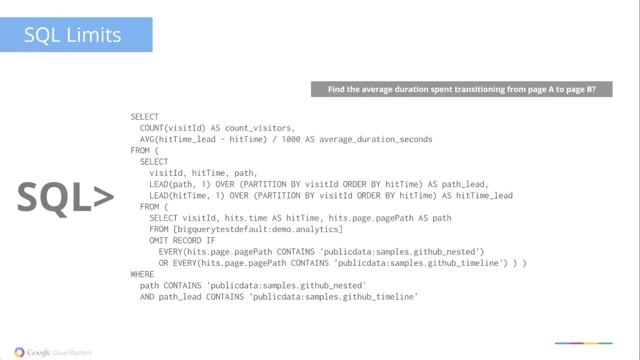 this was significantly more complicated than I was actually expecting, So I apologize. this is a bit of an eye chart, I realize that, But I wanna go through the specifics here and explain how this actually works. So in the innermost query here we need to pull out the visit ID. 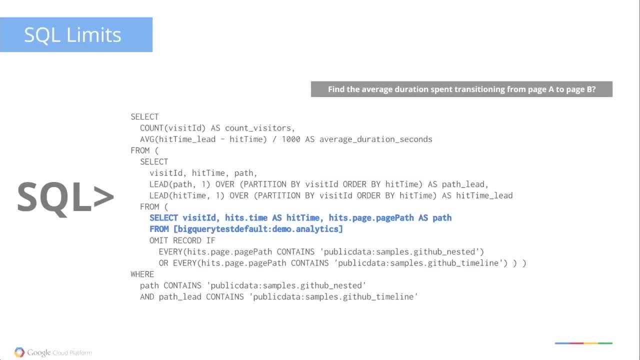 the hit time and the actual path that it was navigated to. The next bit of syntax is omit record. if It's actually something I wasn't even familiar with prior to trying to work on this example, What it does is, rather than just apply a standard where clause 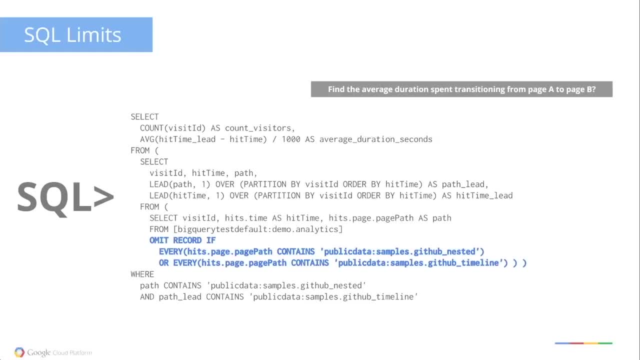 omit if allows me to find rows in which, embedded in that repeated field of hits, both of those conditions. Both of those conditions have been met. In this case, the user had navigated to both GitHub nested and GitHub timeline. So now that I have at least the rows that I'm interested in processing, 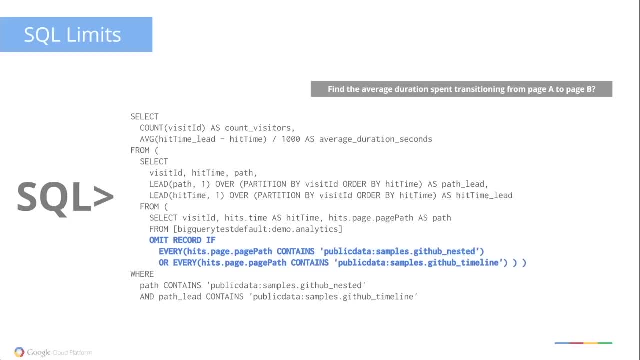 I need to find those cases where they actually did transition between those two specific tables. So I come here and I use one of those analytic functions- Combination of partition by ordering on hit time- and this notion of lead- And what it's essentially doing is it's transposing. 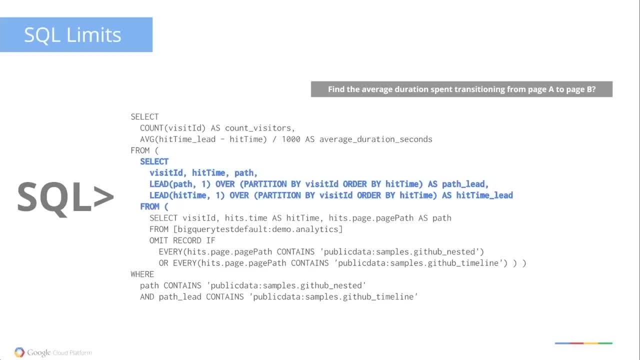 It's taking hit number one and it's transposing hit number two alongside of it, And so on and so forth. Once I have that created using path, and now path lead as the two fields, as I've named them, I can now apply this, this finer final outer select. 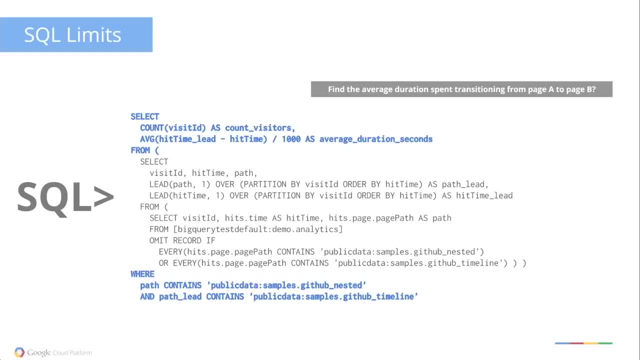 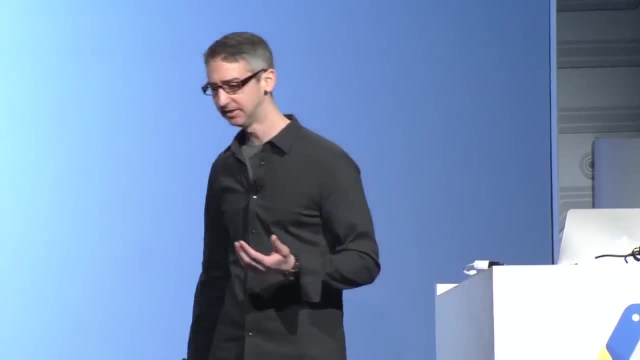 First it's filtering, of course, and it's looking for where path is GitHub nested and path lead is GitHub timeline, And then I can do the count and the average. So this works. This definitely works. There's there's no doubt about it. 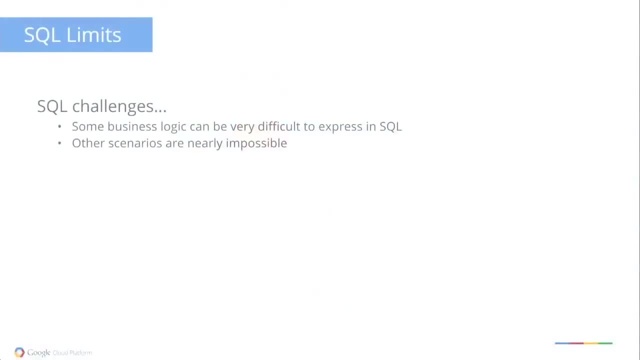 And you can construct all sorts of amazing things, especially if you've been using SQL for years. I would argue clearly: SQL has some challenges. I mean these limits, you know if, if not nearly impossible, in some cases are truly impossible. 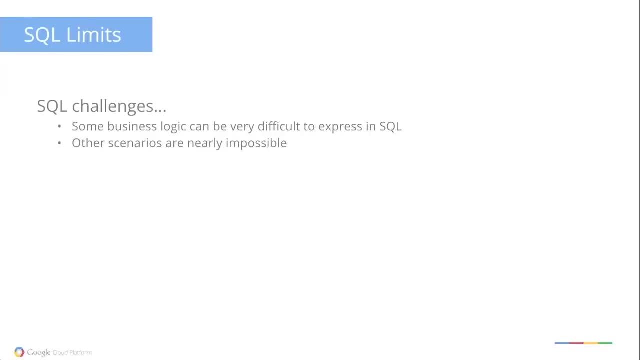 And so I don't think this is anything new. I mean, other databases have solved for this right. There's PLSQL, there's T-SQL. This is. this is pretty standard in the industry. People have accepted that sometimes a procedural language makes life. 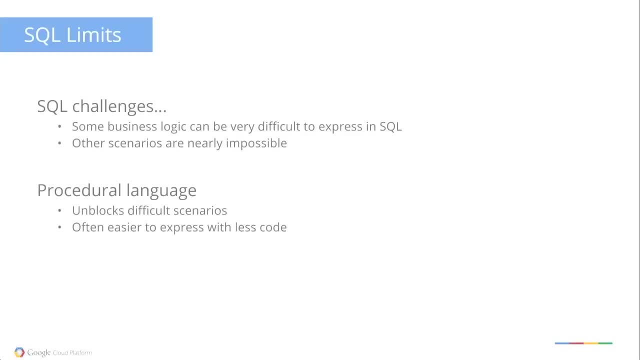 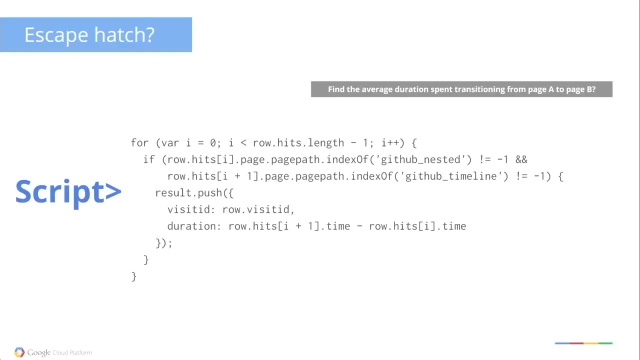 a thousand times easier, Even if you can express it in SQL. it might be that much easier to express your business logic in a procedural language. So what would this do? It's a good question, So what would this one look like? 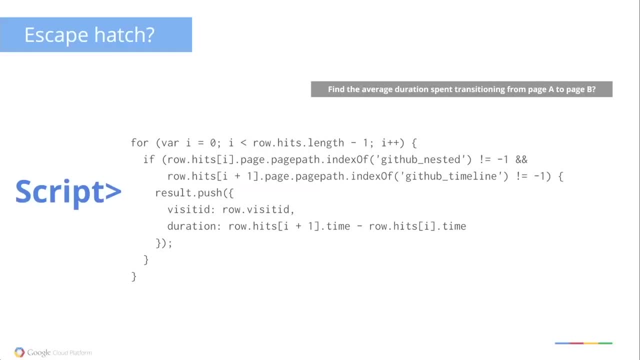 If I just want to find those hits, let's isolate in on that most important part. It's super straightforward: For each row here I have an array of hits. I just need to check if hits sub i is equal to GitHub nested and. 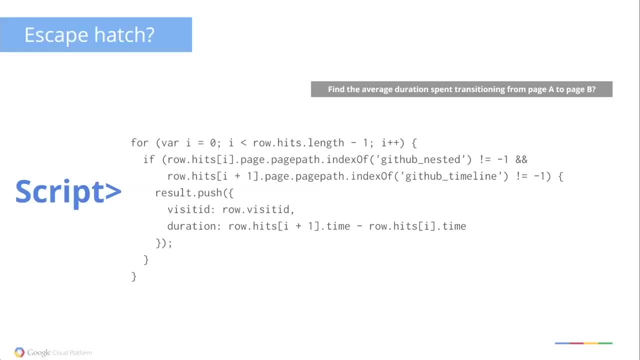 hits sub i plus 1 is equal to GitHub timeline. then do something. In this case, I'm adding it to an array and emitting it, So it's clearly a lot easier, right? I need this escape hatch. I need this ability to be able to go operate in more arbitrary ways. 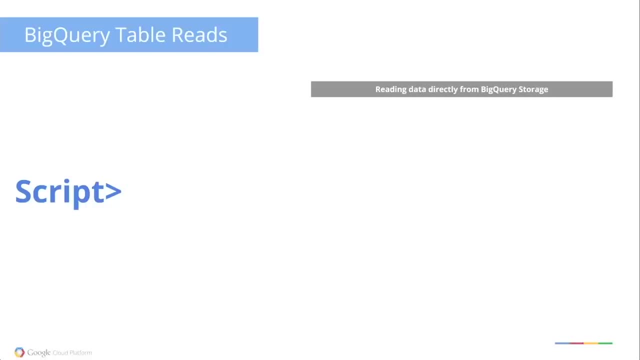 than I can express in SQL in some cases- And I mentioned earlier that you know I don't have a lot of time, right, I don't have a lot of time, But I wanted to make sure that we make this possible. 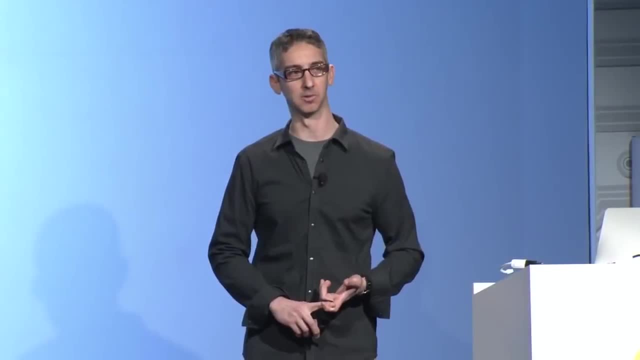 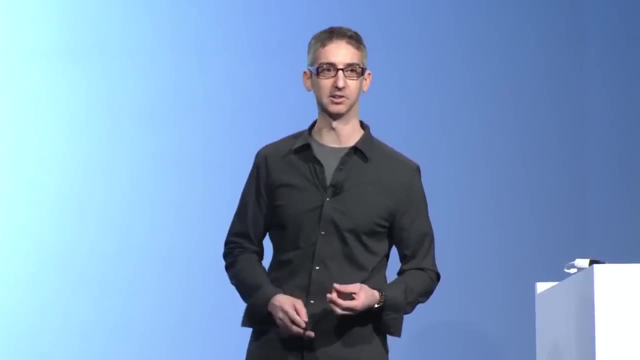 You can do reads directly from BigQuery storage without running a query. In fact, I noted that Motorola was actually doing MapReduces over BigQuery storage. So what we're announcing as well today is not only can you do those reads, but you can now do them at incredibly high throughput. 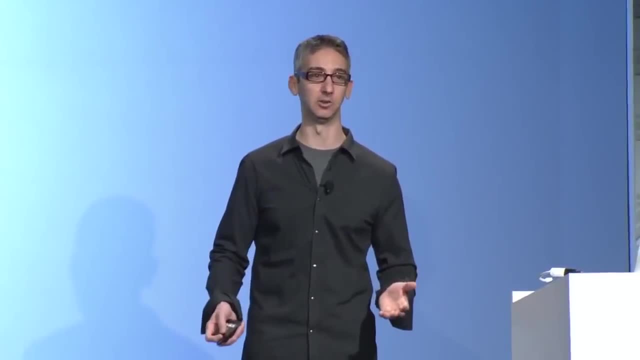 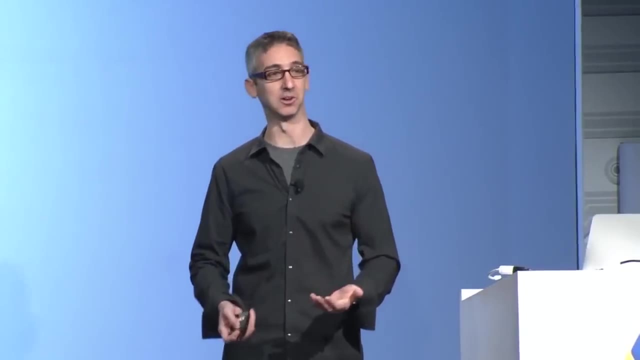 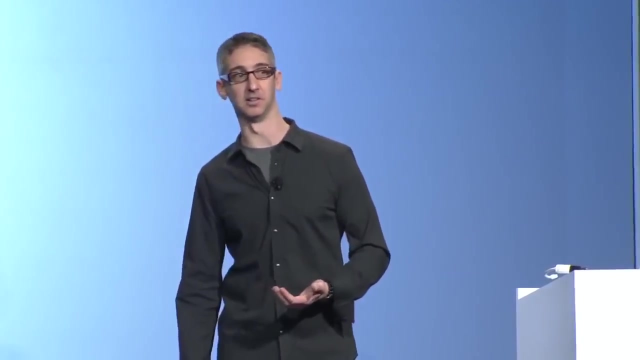 We're making it possible to read in parallel across a huge BigQuery table via Hadoop, via whatever parallel processing tool you have of your choosing. The pseudocode here I've included. But it's trivial to set this up. You first need to instruct BigQuery via an API call that you want to read in parallel. 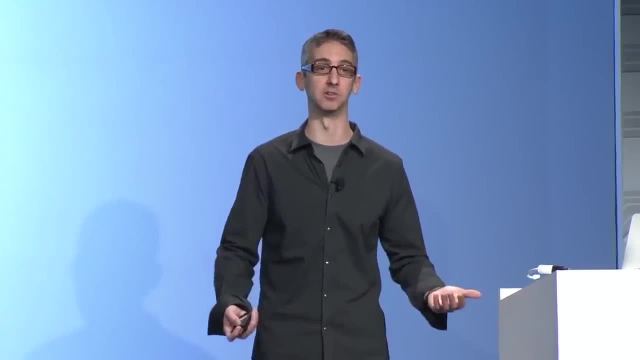 across a given table. You tell us the number of workers you're going to have. Maybe you're going to run 100 MapReduce workers. You then wait for that job to start. Should take no more than a few seconds, And then you would iterate. 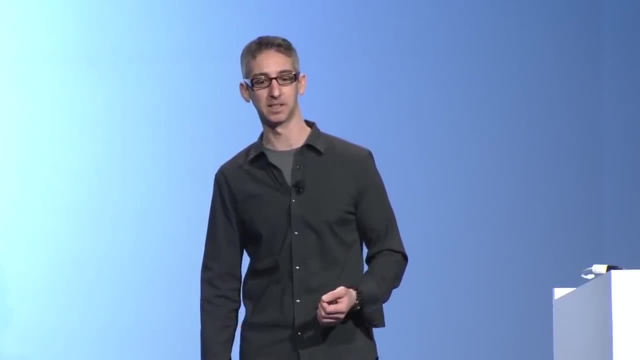 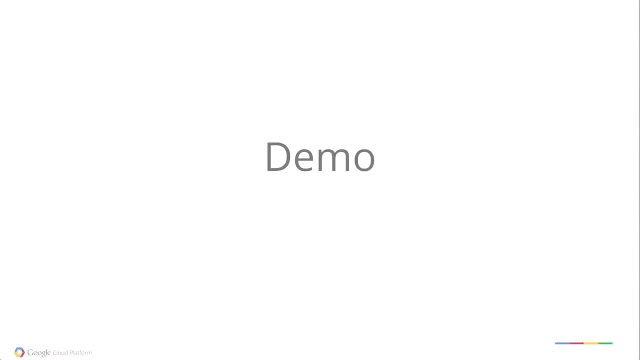 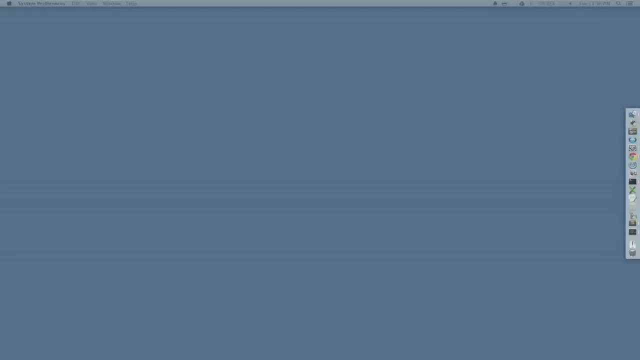 Each partition can be consumed in parallel across that table, So this unlocks a whole new set of use cases. But maybe there's an even easier way And if you could switch to the demo please? Apologies, it's pulling up the wrong desktop. 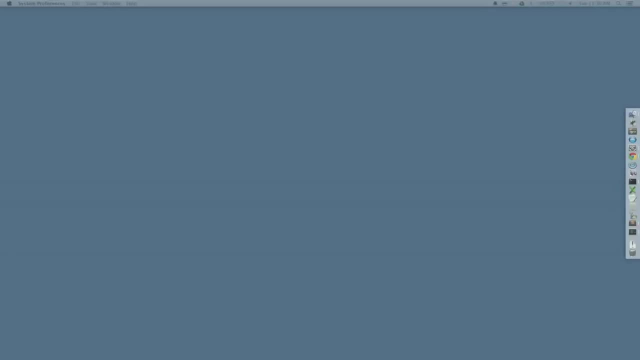 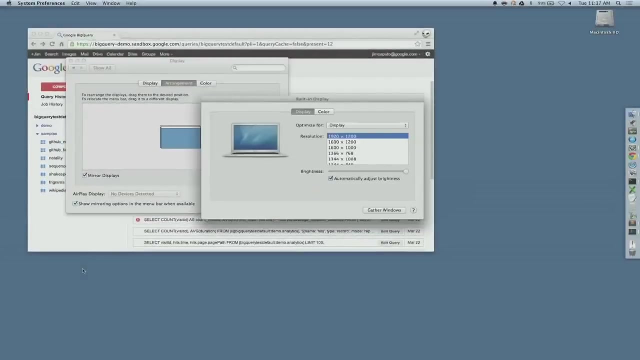 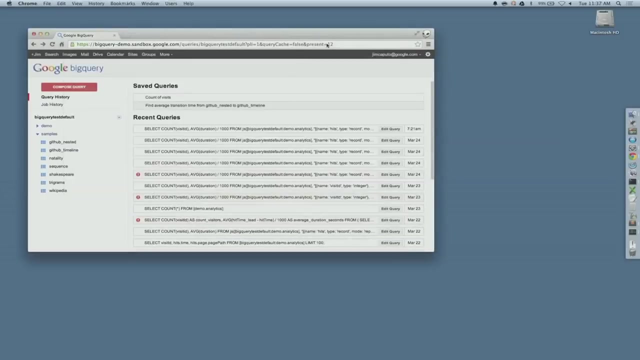 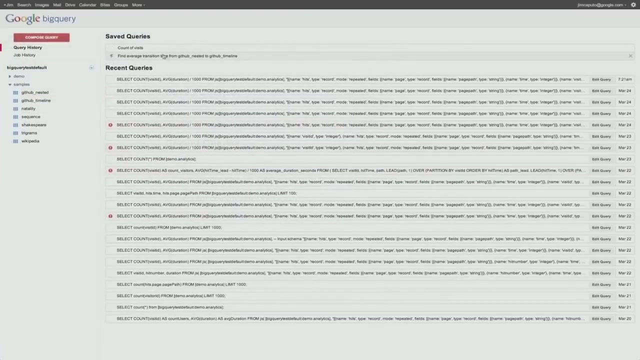 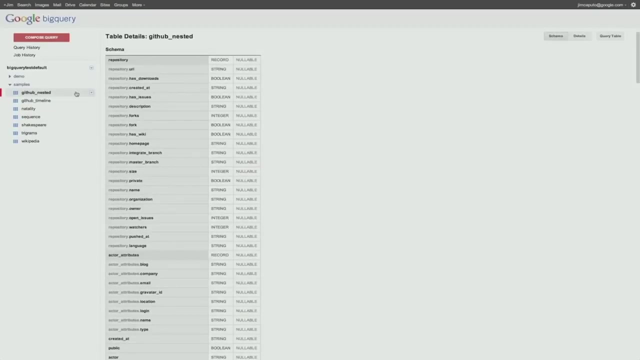 So I'll just stop there. Okay, Turn it off. Okay, The question is, which one? A little help, I'm on desktop 4.. How do I get to desktop 4?? Much better. Hopefully you all can read that from the back row. 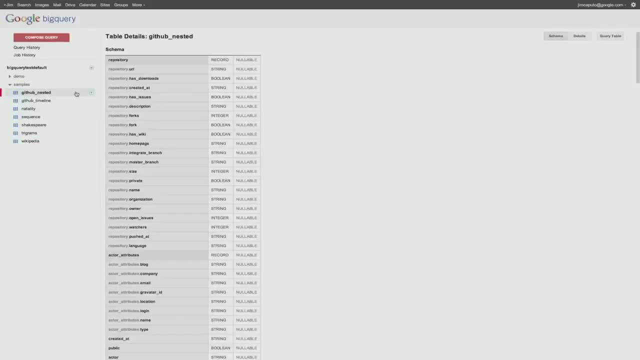 It might be a little bit small. Okay, so what you're looking at here? I mentioned we have the GitHub nested table. This is inside the GitHub timeline table. So here I just induced this behavior. I've navigated between the two. 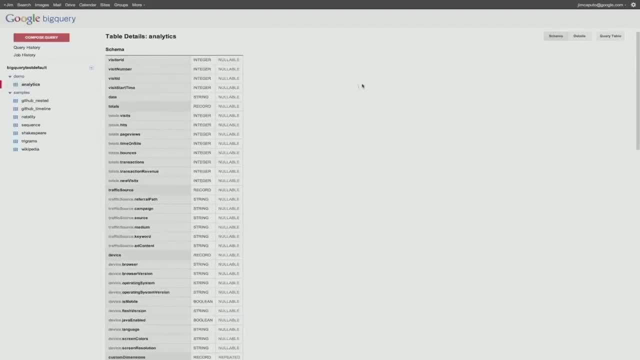 And I've pulled in all of our analytics data to this test Data set here So we can take a quick look There as well. So we have visit id and visit Start time, like i was talking about A whole bunch of other fields here. 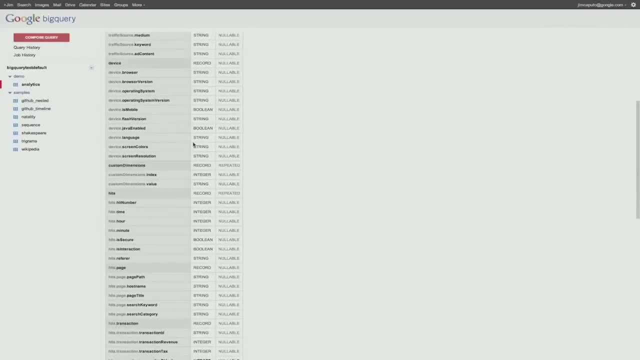 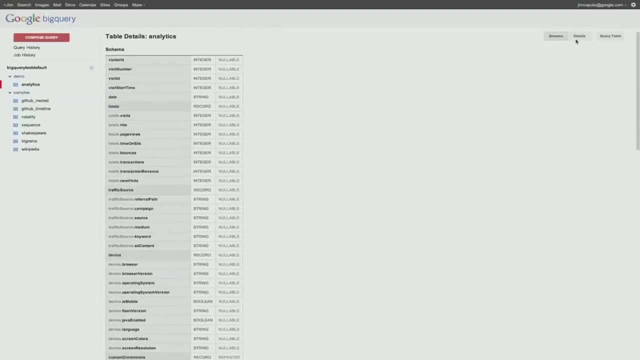 Totals, traffic, source, the device that you've navigated From, as well as that repeated field of hits. So hits and the hit time and the page path. This table isn't particularly large here. It's about 18 gigs, about 11 gigabytes. 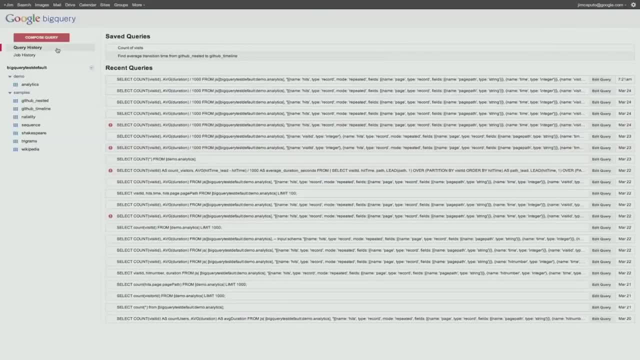 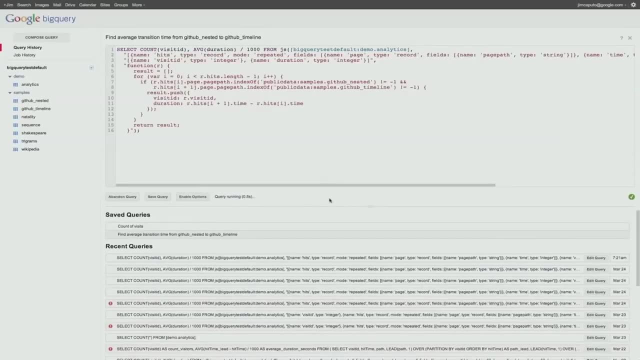 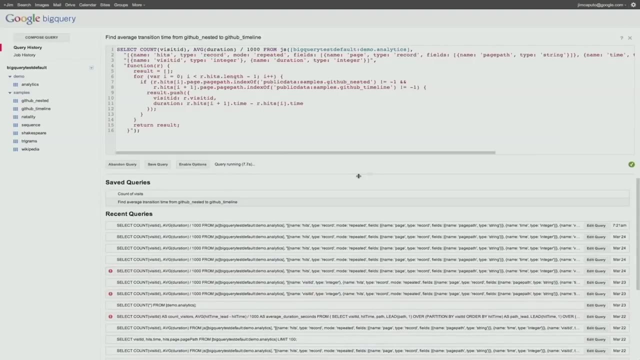 So I mentioned there might be an easier way. Well, indeed there is. We are combining the power of that procedural language right Inside the power of big query, the full scalability of big Query, allowing you to merge right together both sql and Javascript at the same time. And like that i've run that. 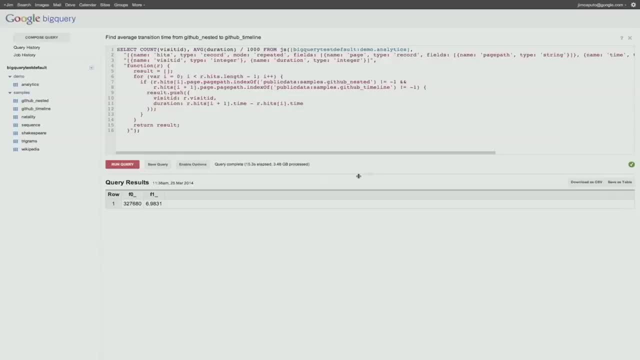 Exact same query now directly inside of big query, Without any effort in terms of spinning up resources, Provisioning hardware, doing any kind of software provisioning As well. So taking a closer look here it's pretty straightforward. We've got a standard sql select at the top here, pulling from 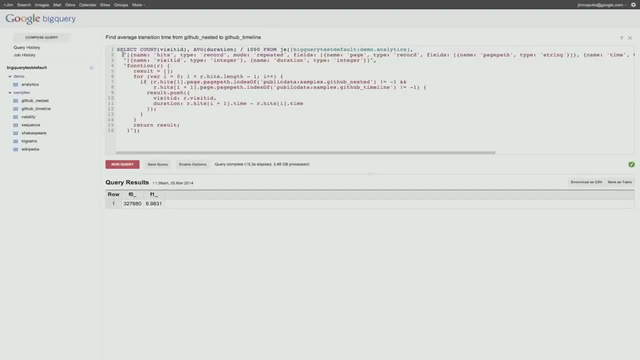 That given table The next row- i'm instructing, Big query: what is going to be the input schema i'm interested In? So which fields do i want to pull Out of that table? the following row is: what's the Schema that's going to be emitted from the function and 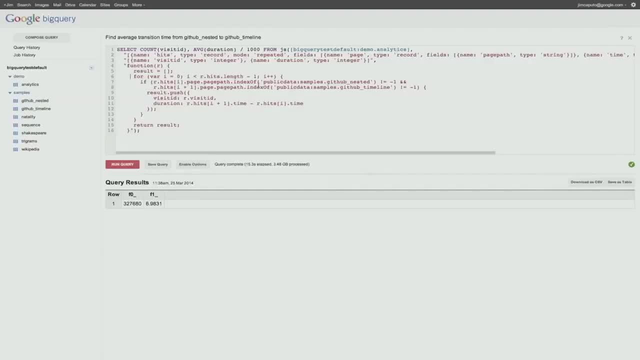 Then, as you can see the function itself, And i would argue, going back to that, can you push the limits With sql? what are the boundaries there? Let's take a slightly different example. Maybe i don't want to look specifically at that transition. 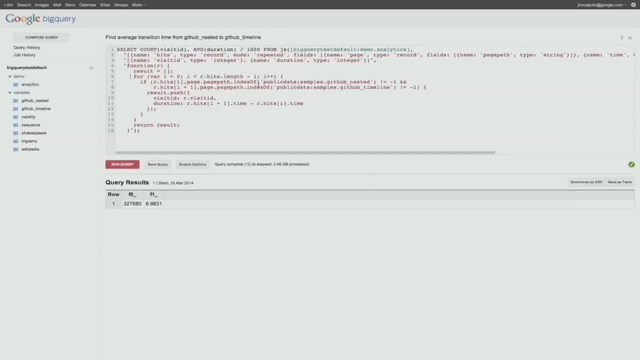 From github nested to timeline immediately, but i'd like to see If they skipped a page or two in between. So changing that is as simple as coming through here making a Quick update. It's very easy, at least for me, To understand this. relative to the challenge, i think i would 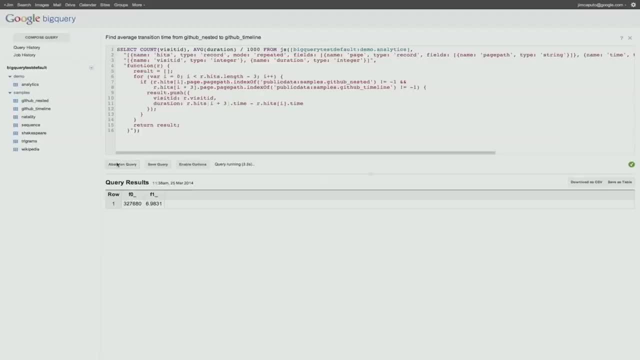 Endure, So i'm going to go ahead and Try to figure out how to do this in sql. So off it runs. This is coming soon. We're going to make it available to you. Excuse me, please contact the sales rep to get started. 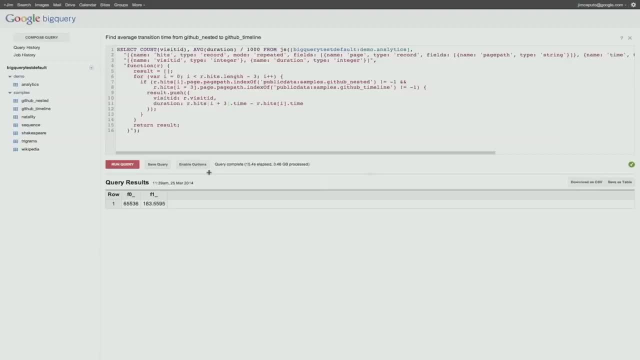 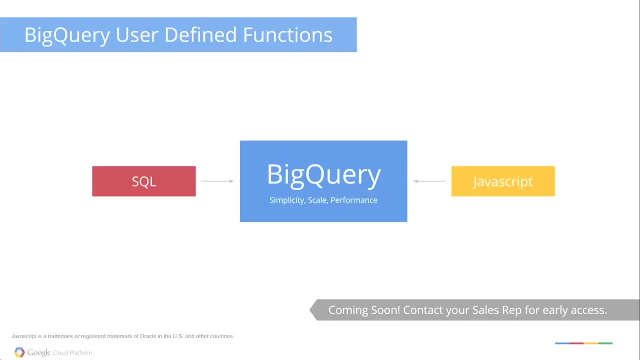 Hopefully this one will finish here in a moment, And indeed it does. Please let's switch back to the Slide. So with big query and the Combination of both sql and now javascript, udfs, we think we're Unlocking a whole set of new use cases. 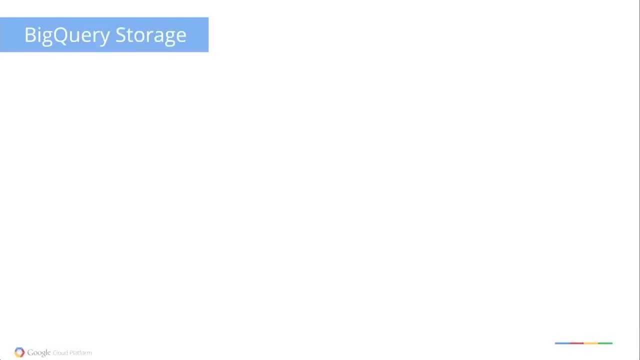 We're very excited to see what you guys can come up with next On this, So big query storage. In summary, it's optimized for sql, of course, and we're going To continue to invest there. We have a whole bunch of new. 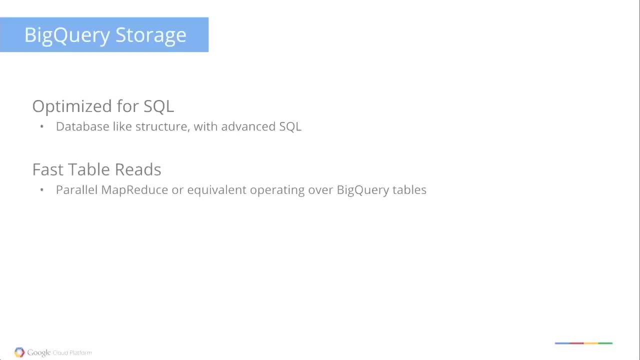 Improvements coming down the road. Fast: table reads: a new ability To do huge scale map reduce directly against a big query Table, not having to necessarily do any operations in between. And finally coming soon, javascript udfs on top of big Query data directly. So the last area i wanted to come. 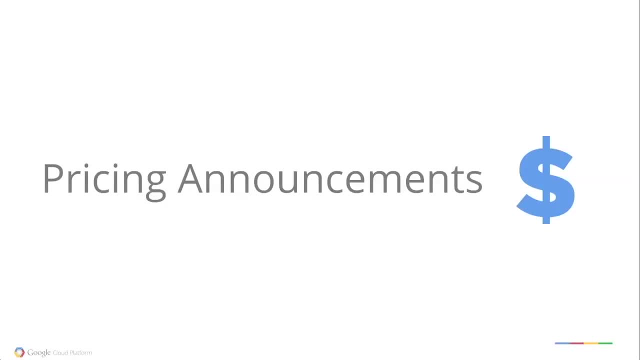 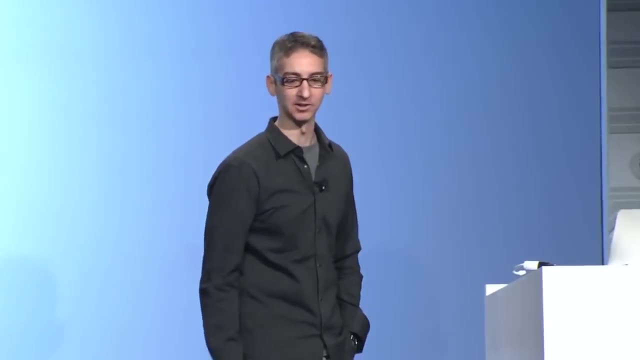 Over are those pricing announcements. We talked about those this morning in the keynote. We're definitely excited about opening this up more broadly To more users. So why are we doing this? Well, of course, to reduce price, lower barrier to entry. 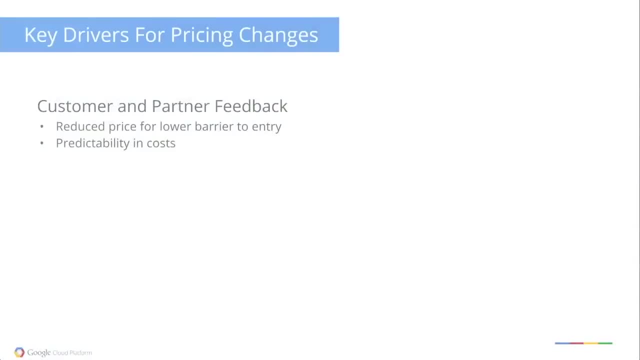 We want more people. We want everyone to have access To big data processing. We've also heard from the Larger customers. we have that really wanted: predictability in Terms of cost. Additionally, we've seen these New usage models emerging since we started. So data warehousing, now streaming ingestion, doing real 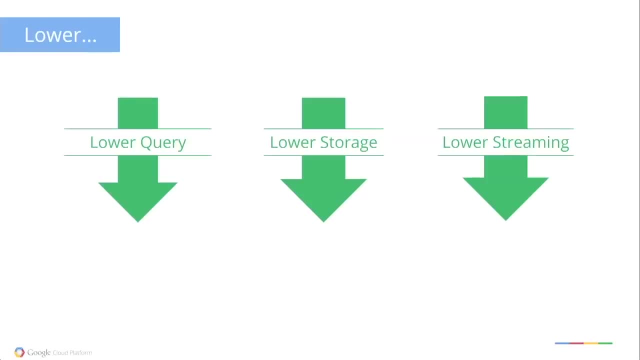 Time. capabilities And udfs coming along, So lower across the board. everything is coming down. So lower: query pricing: $5 per terabyte, an 85% reduction off Of our current $35 price point. Lower storage pricing: $26 per. 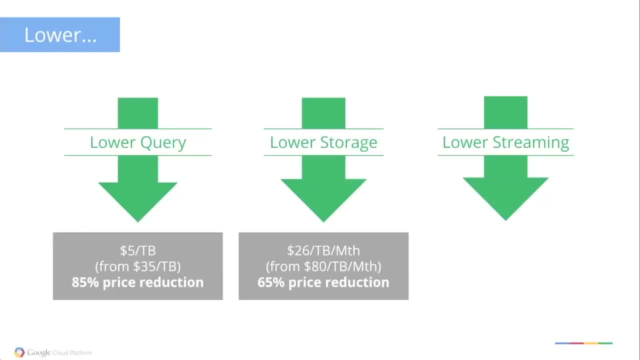 Terabyte per month, 65% reduction. And what's really important to Note here is that your storage pricing is completely independent From your query pricing, So you can park as much data as You want with us at bare bones pricing and not necessarily have 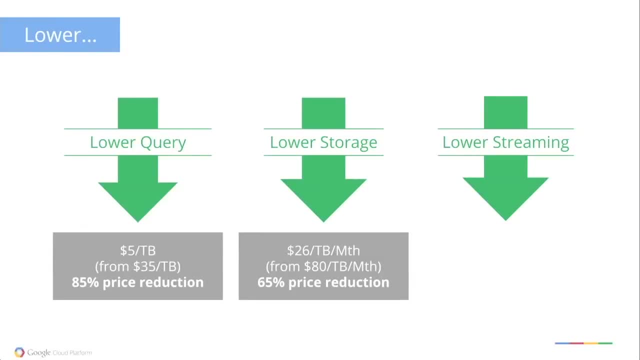 To pay a dime in query costs. Use it as much or as little as You want in terms of query, It's immediately available. Only google has the infrastructure, in terms of storage, network and Query capability, to give you these things independently. And finally, lower streaming costs: One penny per 100,000 rows. 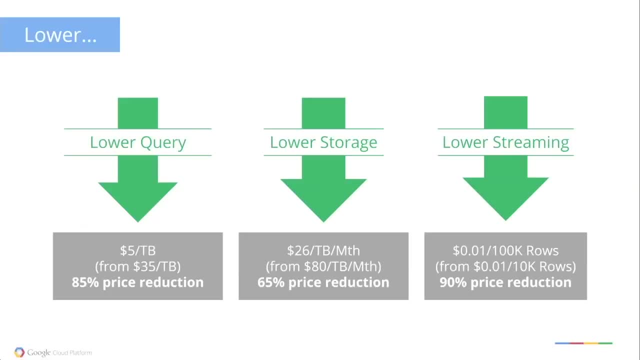 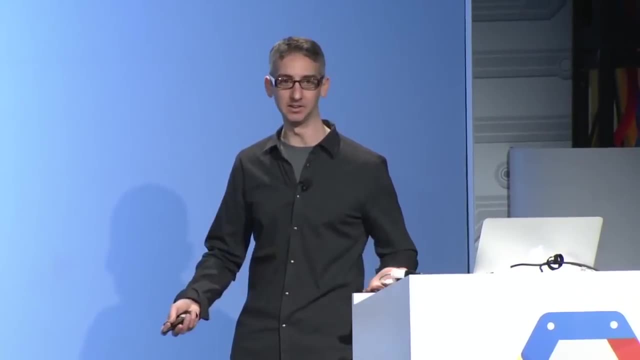 We've actually deferred pricing on this until july. We'll let you get started now. So on-demand query pricing. a Closer look at this. This is essentially our existing Usage model. It's ideal for interactive ad hoc analysis. It leverages a very large shared pool of resources. 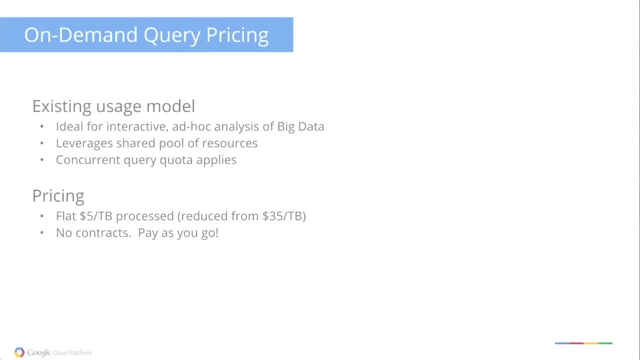 Because it is a shared pool, we do impose these limits in terms Of how much a single user can use, making sure everybody gets Their fair share of those resources. Pricing is simple: $5 per terabyte processed, no contracts, pay as you go. 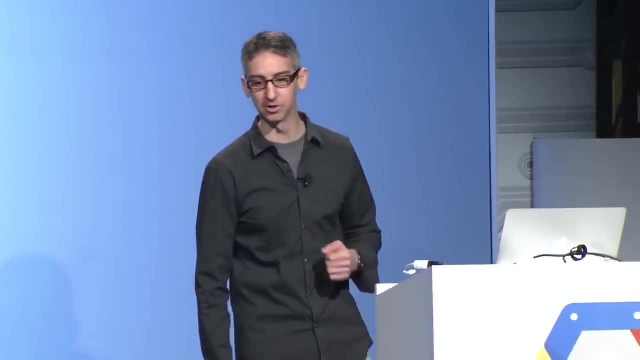 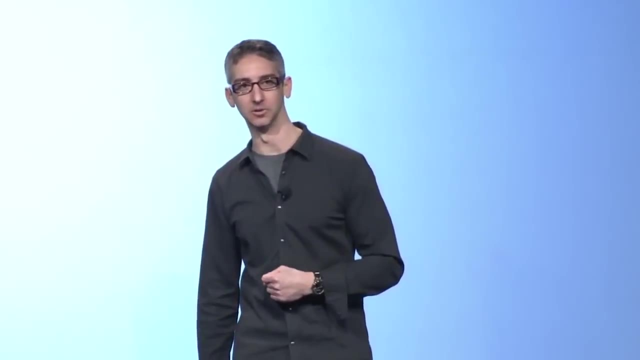 It doesn't get any easier, But it was also mentioned this Morning. we have a whole new pricing model coming online. It's reserve capacity, It gives predictable costs for Those larger workloads, Consistent performance and we Remove those concurrent query quotas. You choose how much capacity. 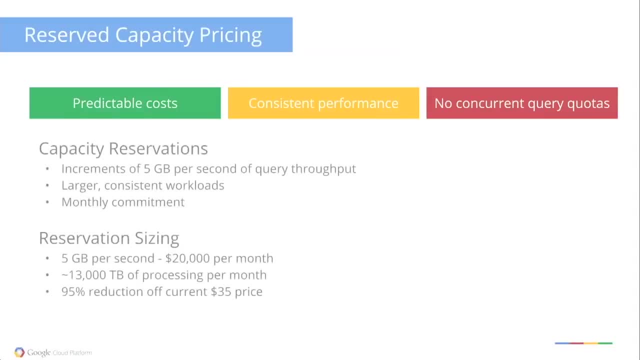 You need to send as many queries as you like. So capacity reservations, The purchase in increments of Five gigabytes per second, Something that's relatively easy To get your head wrapped around. How much do i want in terms of Throughput, not how many machines do i need? 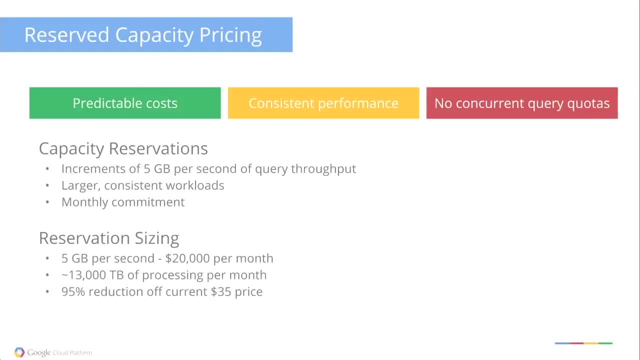 To buy. how many cores do i need? do i need ssd versus Regular disks? what do i need to do? Larger, more consistent workloads is what this is after, Obviously with a monthly commitment attached to it. Each five-gigabyte-per-second query quota is going to be. 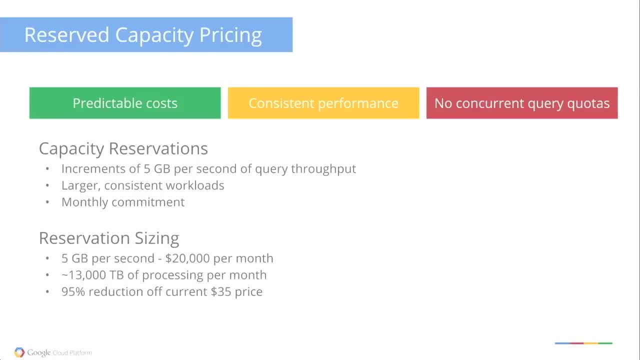 $20,000 per month. It enables 13,000 terabytes of Processing per month. If you were to fully utilize That, that's actually a 95% price reduction off our current $35 price point. So what is 13,000 terabytes? 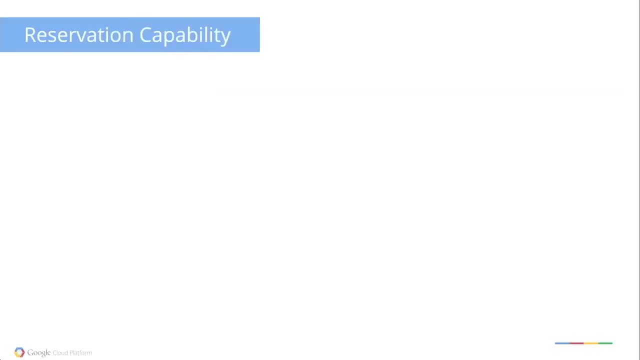 Though that sounds big, but i'm not Really sure what it means in reality. So i put together a quick example customer scenario here. Let's imagine you have 50 terabytes of data stored And your average query size is about 2.5 terabytes. 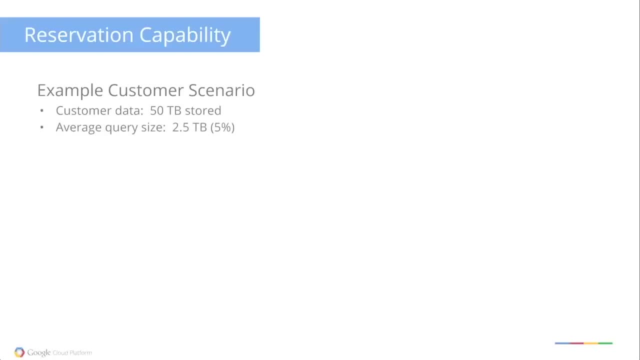 So you're going to have a lot of data stored Right off the gate. you might question: why just 5% of my data? Why is it so small? well, i mentioned earlier column Under data format is very highly optimized. 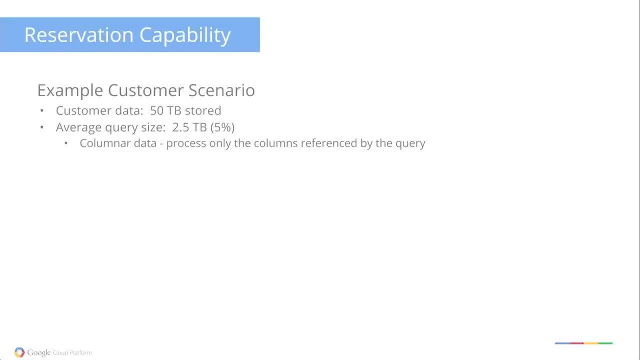 We reduce the amount of data scanned simply based on the Columns referenced. So if you had 50 columns in the Table and you're only referencing five of those, Probably about 10% of your data is actually going to be scanned In that query. But there's other places you can. 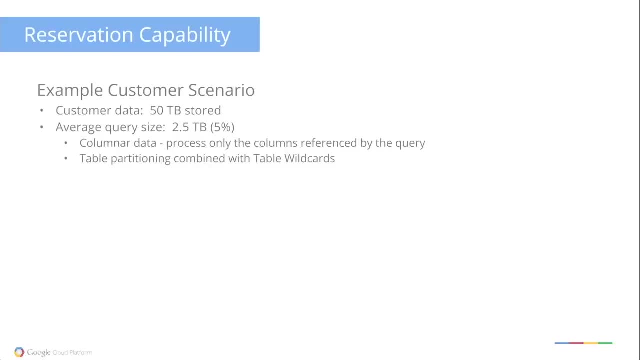 Save So, table partitioning and using Table wildcards. If you have daily tables and You only need to query over seven days, then only reference Seven days' worth of data. You don't need to reference the whole Year Or, additionally, table decorators. 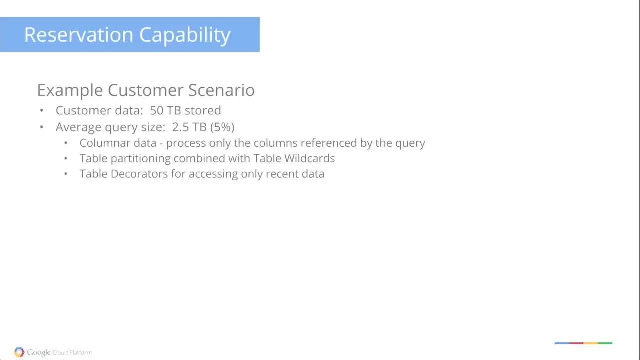 If you're doing more recent information that you want to Pull out via the streaming api, So there's many ways in which You can get there. In fact, a lot of our customers See a lot lower than 5% in some of their use cases. 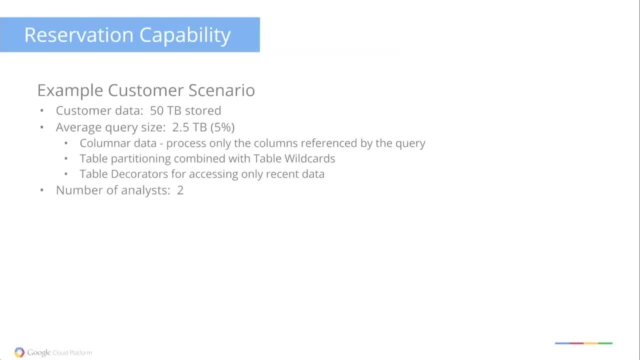 So i'm also going to imagine that this company has two Analysts that they want to have operating on this particular Dataset And those analysts are going to Run about 75 queries per day. So in total that's 2.5 terabytes. 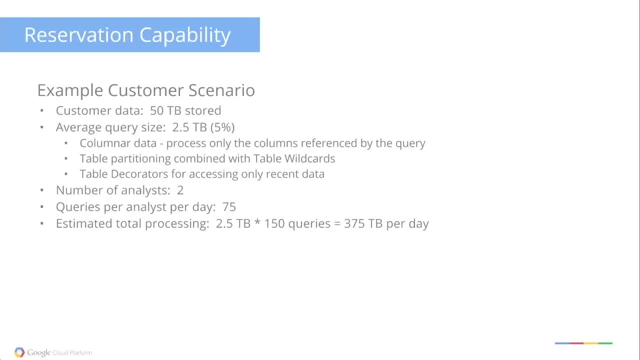 Times 150 queries, about 375 terabytes of processing per day. As it turns out, our smallest reservation can accommodate a 50-terabyte dataset, Because a single reservation of Five gigabytes per second enables you to do 432 terabytes. 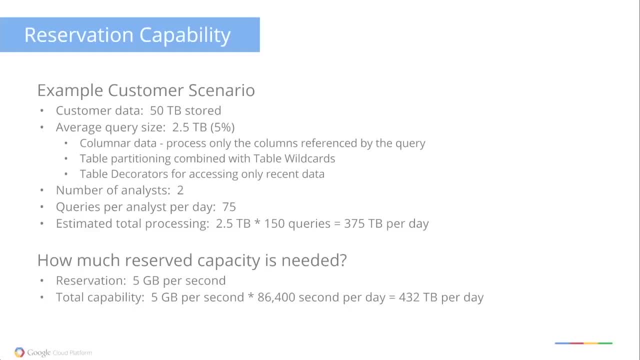 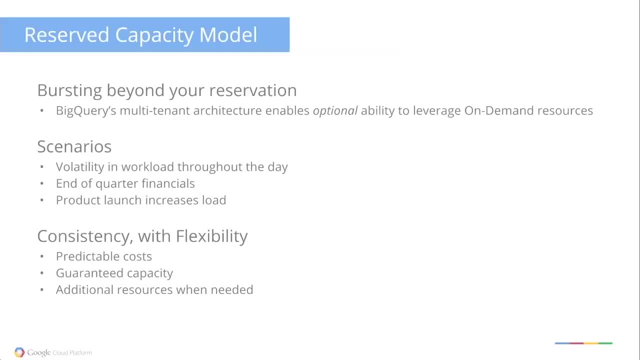 Of processing per day, So quite a bit of capability Just from the smallest reservation increment. The other thing that we enable, because of big query's multi Tenant architecture, is the ability to not only use your Reserve capacity but optionally burst into our on-demand. 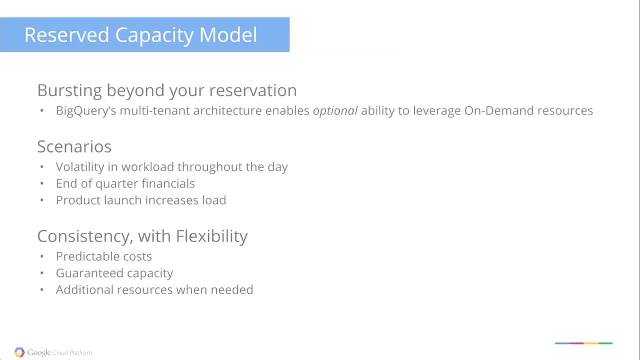 Resource pool. It's just something that we Are capable of doing. The scenarios here are endless, So it might be just during the course of a given day. there's Volatility in your workloads. You want to have the ability to Spike and not necessarily have all of your users backed up, and 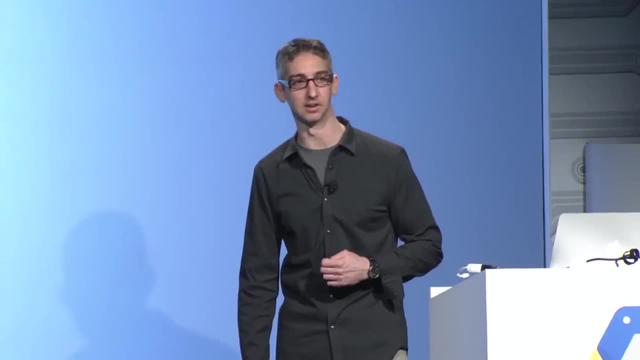 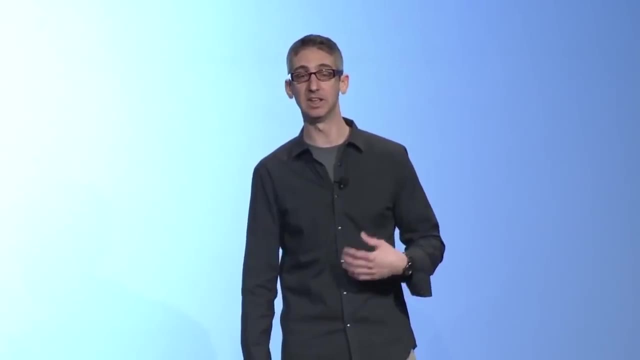 Waiting, Or maybe the finance team is Struggling to get financials done at the end of the quarter, Or maybe literally you're just increasing your volumes that Dramatically and you haven't figured out how much more you Want to provision. but you need the capability to run more. 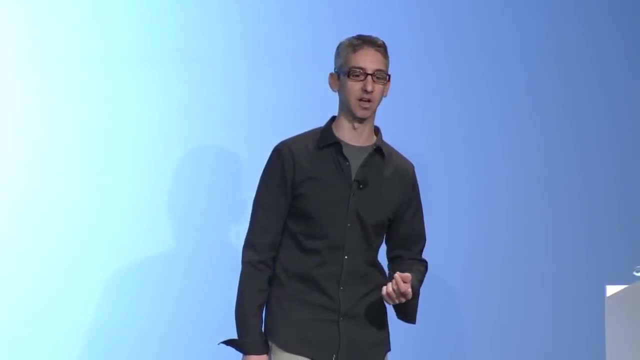 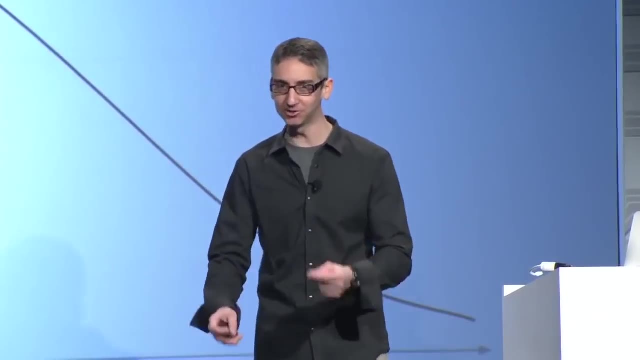 Queries. So it offers that predictability And cost with guaranteeing that you're going to be able to Provide guaranteed capacity and additional resources when you Need them. So what does this actually look Like in practice? this is going to get in depth With some charts here, but this should be fun. 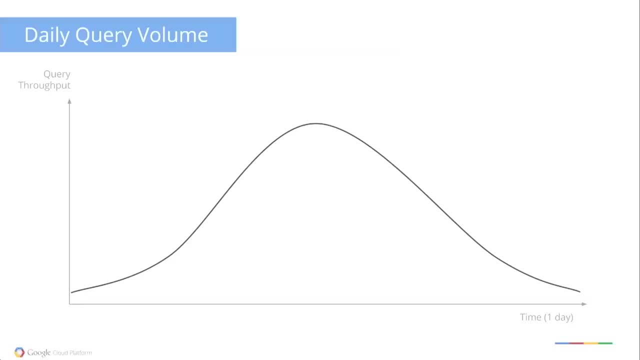 So here's a given day's worth of volume, And you can imagine it wouldn't be a perfect bell curve, but, as You might guess, the volume is going to increase during the Middle of the day for a given work day, right, And so this curve is measuring query throughput. 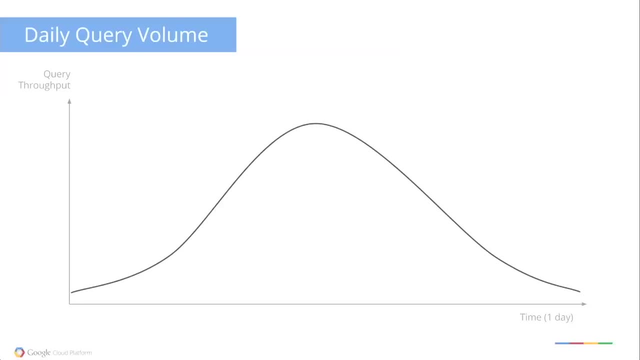 Essentially the number of queries you're pushing into the System at any given time for your reservation. In this case, using that customer example, the total Query processing during that day was 375 terabytes, So that customer reserved five gigabytes per second and they. 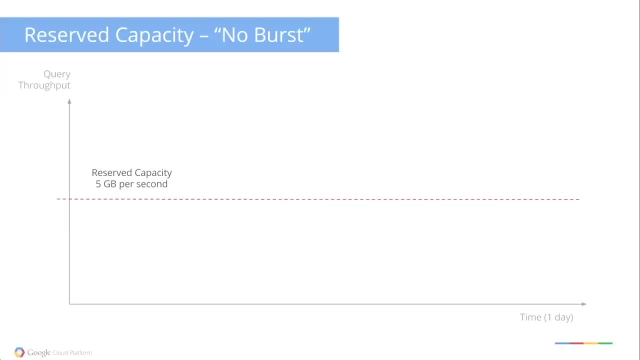 Chosen not to actually burst. That's where they started out. They felt like that was the appropriate approach, And this is what you would get if you were provisioning your Own hardware or buying or reserving n number of instances. You would get something that looks like this: 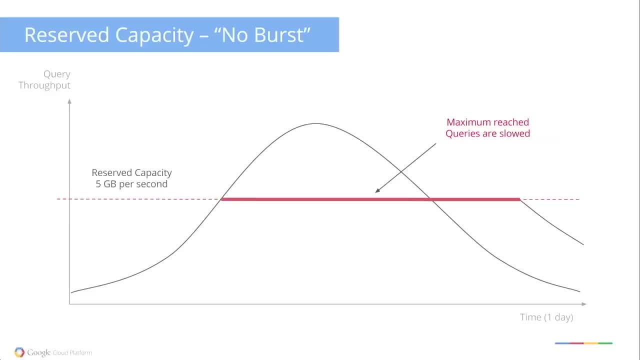 Rather than the smooth bell curve, you would end up capping Your capacity. All of your queries would start Slowing down, Your users would get a worse Experience And then, hopefully, at some point Near the end of the day, the system catches up and recovers. 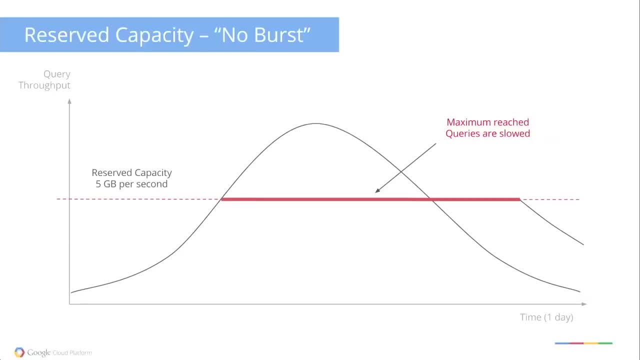 In the middle of the night and eventually you come back in the Same experience again. We've all experienced this. Oh, the sql server is running slow today because there's a Lot of workload going on right, But with big query you don't. 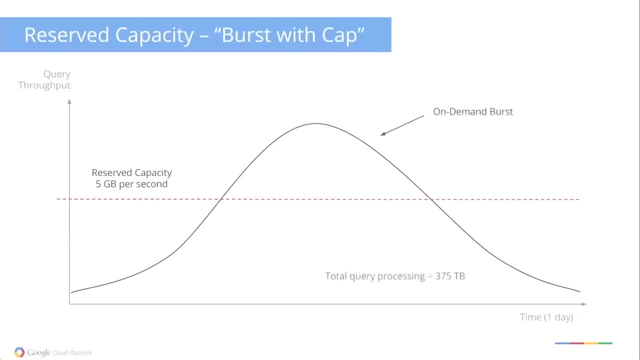 Need to run into this problem. In our case, we're able to Actually burst that additional need above and beyond your Reserved instance. Ironically, the query capacity Required is the same. We still have 375 terabytes of Processing to do in that day. The difference is your user. 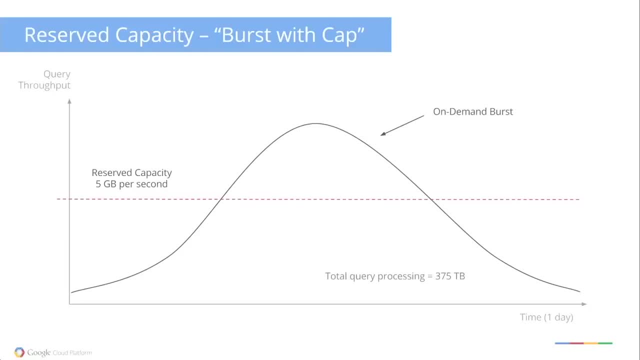 Didn't have to bump into those painful slowdowns. So this is burst with cap. There was no change. I'll explain cap in a moment And the next example. they've Also chosen burst with cap, but over time, their data volumes. 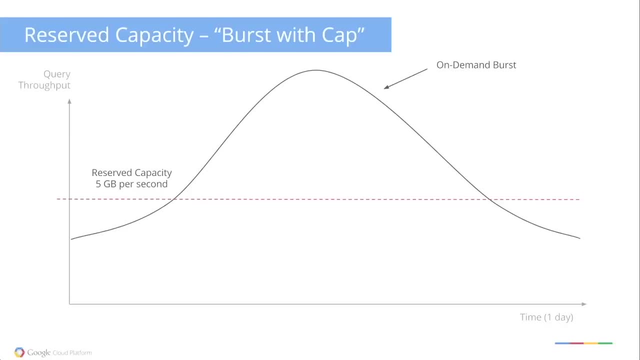 Have grown. The number of queries they're Running is higher, So they're spending the vast Majority of their time above their reservation, more than They've reserved in terms of query throughput. So what happens in this case? because they've told us they 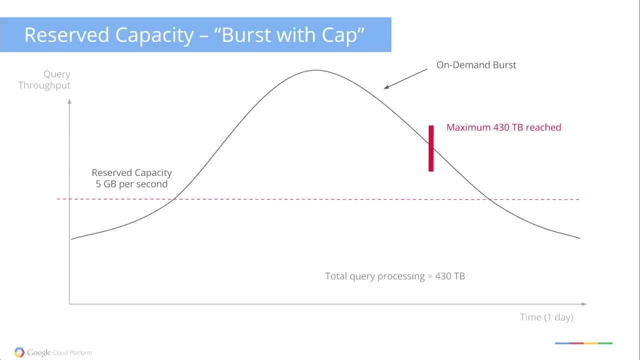 Said we can't go beyond our $20,000 per month budget. we're Actually going to stop them at some point. We're going to stop them technically at 432 terabytes in That given day. They could, of course, go Outside the reservation and still run on-demand queries. 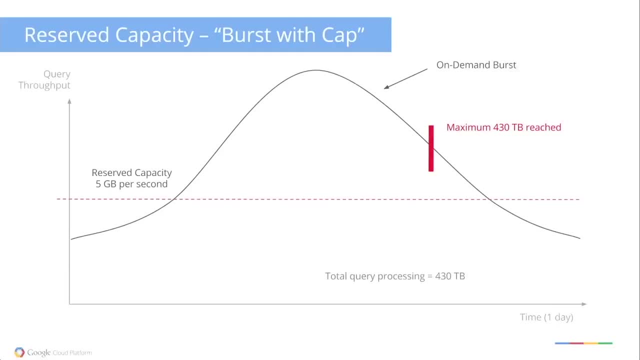 I want to be clear about that. But they have told us, they've Instructed us, they don't want to go beyond that cap. And then, finally, the last example, this case they've Chosen they haven't figured out exactly how much more they want. 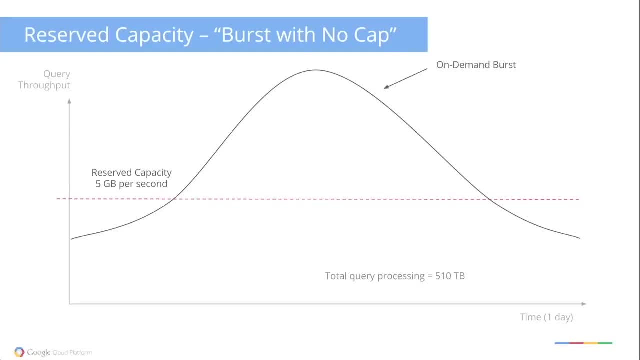 To reserve, but the last thing they want is their queries to Get blocked. So they're allowing this to go Through. They're going to process, in This example, 510 terabytes. So a number of scenarios there, And i realize that might be a bit complicated, but i'm trying. 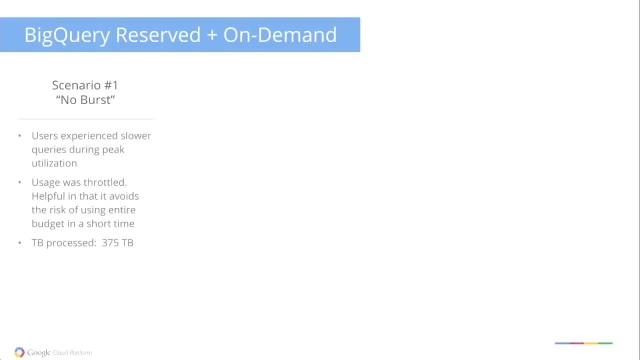 To highlight the tremendous amount of flexibility we're Bringing. The first scenario is perhaps the Most obvious one, because this is what most people face on a Given day. They buy a fixed amount of Capacity. they're capped at that capacity. Perhaps there's some benefit here You would avoid if you were. 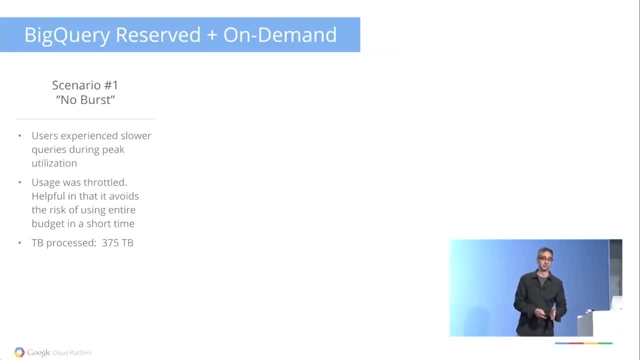 Truly capped in terms of budget. you would avoid consuming too Many resources too early on in the day. The second scenario: they ran over the top of their Reservation, but they still consumed the exact same number Of terabytes of processing, So there was no additional cost. Third scenario: they did a burst and they actually bursted Too far along, But they got more. They actually got 430 terabytes, They told us the cap, so the Additional cost again is zero. And then, finally, in the last Scenario, they ran a total of 510 terabytes, roughly 80. Terabytes more. We multiply that by the standard On-demand rate for an extra $400 that day. So we believe that bigquery is finally realizing the true Benefits of cloud here: Simplicity, the performance you Desire and the scalability you need. 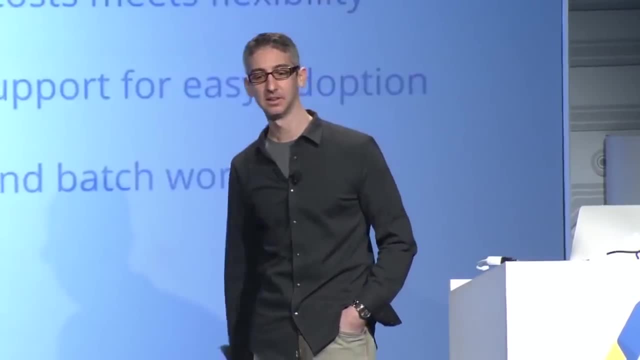 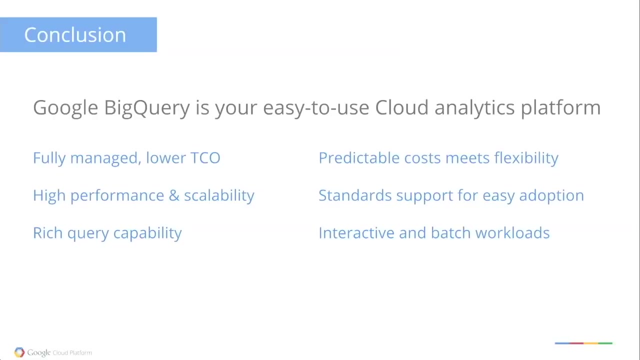 Whenever you need it. So, in conclusion, you've seen a Lot today, both in the keynote this morning and some of these Examples here. We're trying to make it Simpler for you in terms of storage. We're trying to unlock all the use cases, whether it be 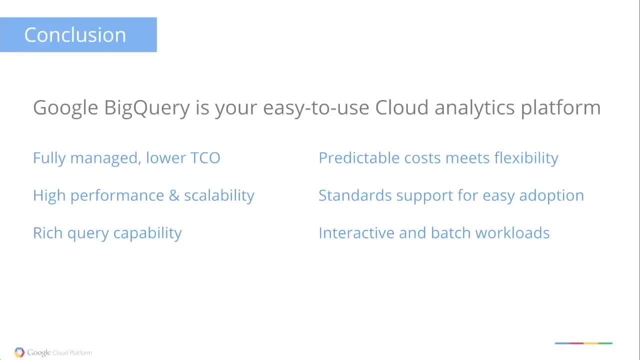 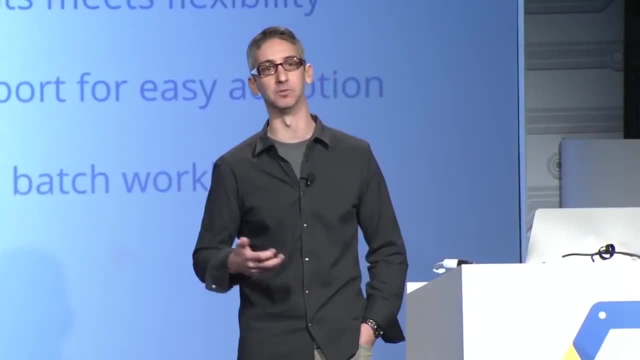 Something you want to power with sql, or something you want to Power with a mapper or, coming soon, sql, udfs, all merged right Inside of bigquery And we've made it tremendously Easier in terms of both cost and provisioning, simplifying the